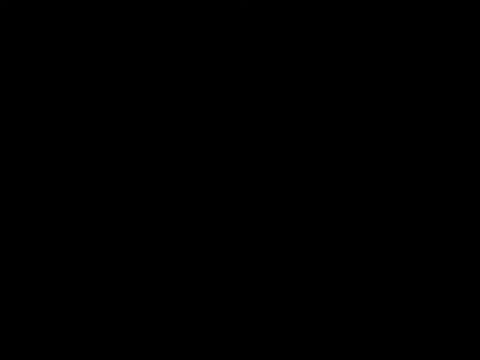 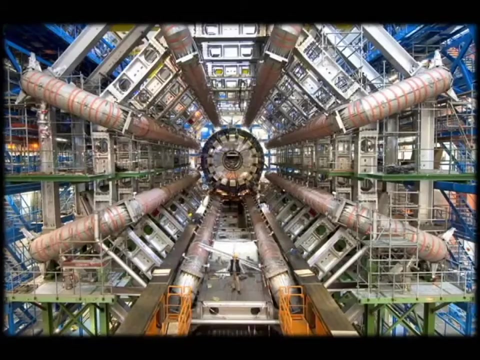 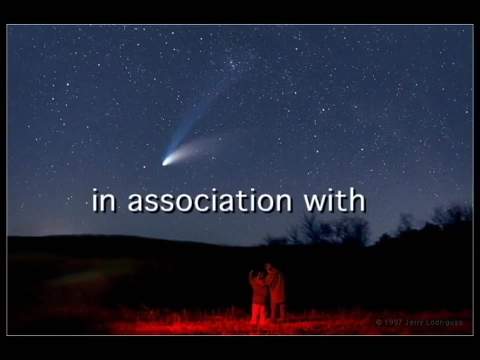 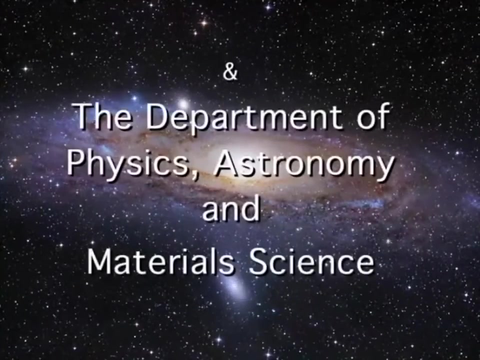 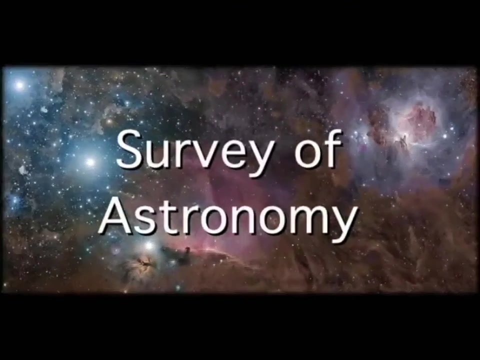 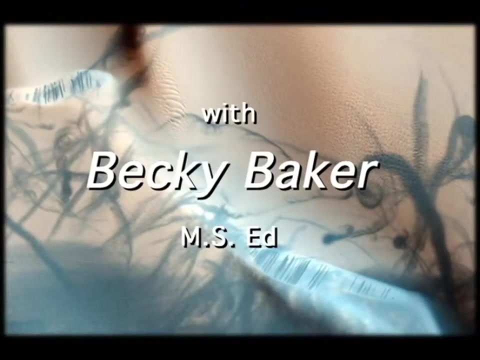 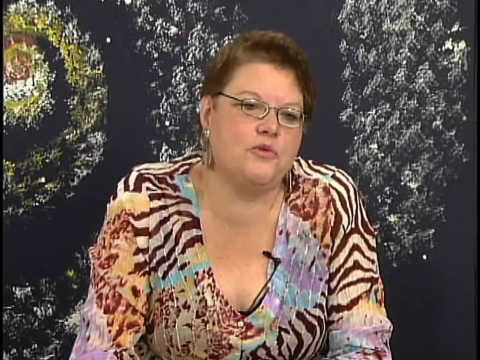 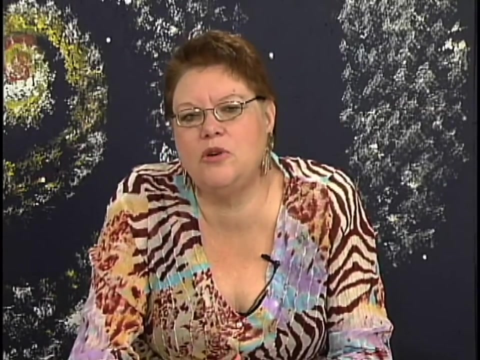 Thank you for watching. Well, welcome to the session today, guys. This time we're going to talk about the moons and the rings. Now I also want you, after we finish this today, to go ahead and head toward Blackboard, because I've got some more in-depth information that we'll put on Blackboard. 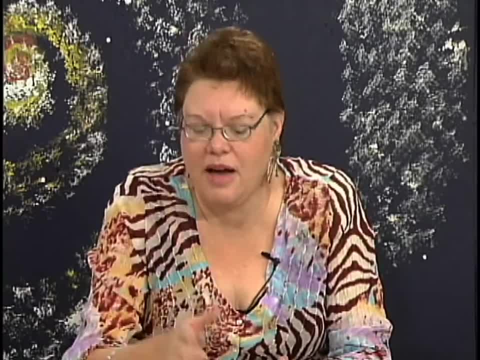 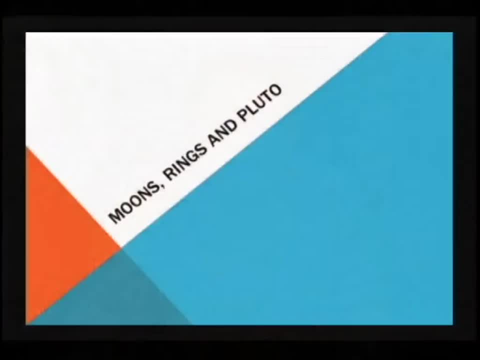 where we can actually start having you guys compare the moons side by side and looking at what's going on. So this I really just want to use as an introduction to the rest of the moons out there in the solar system. So this session, guys, I want to talk about the moons, the rings and then poor little Pluto. 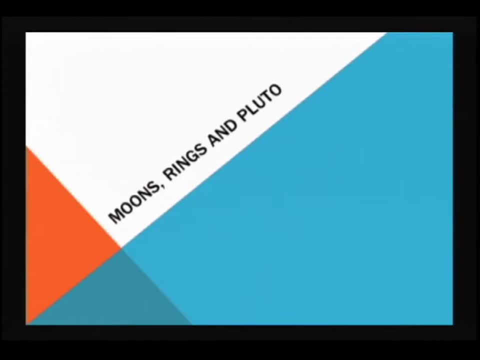 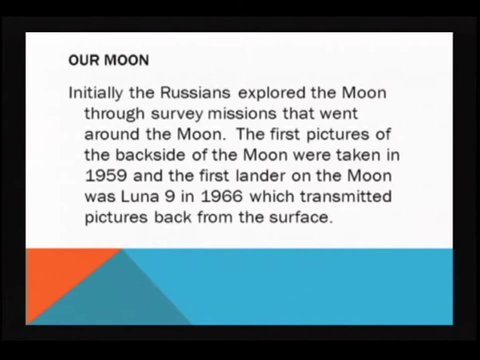 And so why is Pluto no longer a planet? It certainly was when I went back to school many, many, many long years ago. So let's start talking about our moon. Initially, the Russians were the ones that explored the moon. They did that through survey missions that went around the moon. 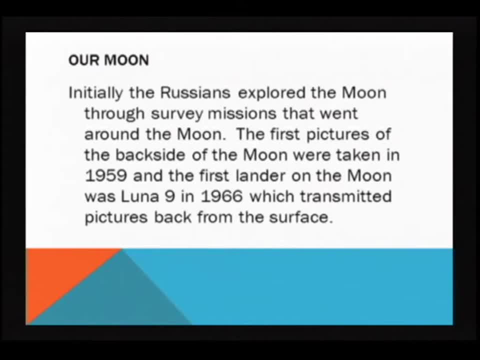 and that's why, when you look at maps of the backside of the moon, a lot of those names are not from the United States. They're from then, the Russians, because they were the first ones that went around the backside, so they got to go ahead and name a lot of the craters and things like that. 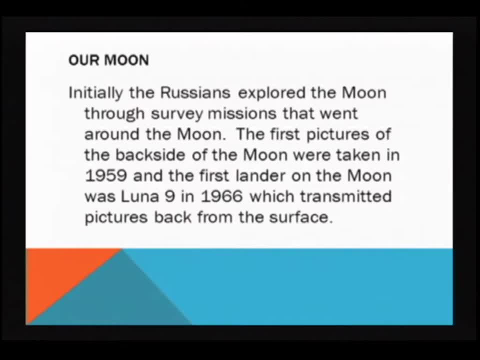 First part of the backside of the moon was taken right around 1959, and we didn't go ahead and actually land on the moon until 1966. And every time we've gone to the moon, gone around the moon, and pictures are always extremely important. 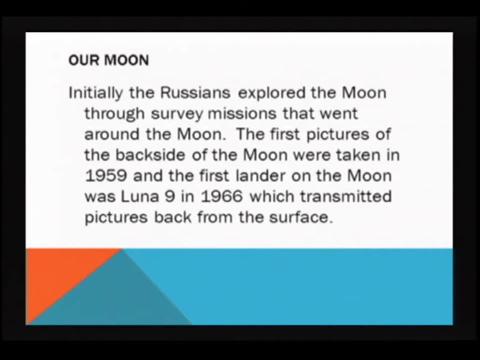 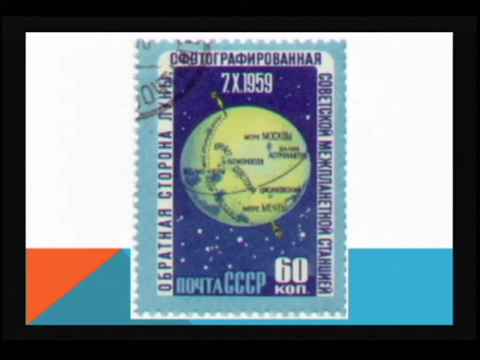 So that certainly transmitted pictures back from the surface itself. And this is a picture of one of the stamps that the Russians produced to go ahead and honor the fact that they indeed were the first ones that went around the moon. And you can see that we're looking kind of not only at the front side there. 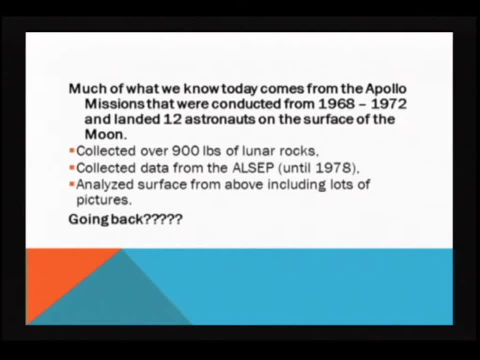 but also a little bit of the backside. We're going to find out that the backside is very different than what the front side is. Now, much of what we know today this is from the Apollo missions, and the Apollo missions were from about 1968 to about 1972.. 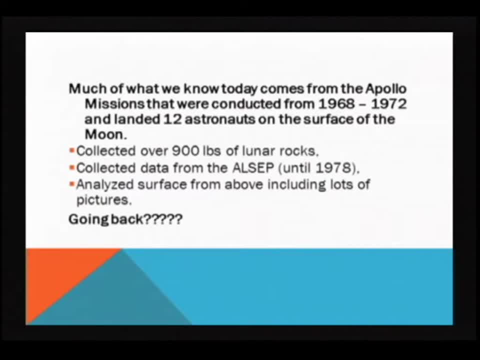 They landed 12 astronauts on the surface of the moon And sorry ladies, unfortunately they were all men. Maybe eventually we, as a female species, will get back to the moon and be able to walk around up there, But we have had 12 astronauts, all from the United States. 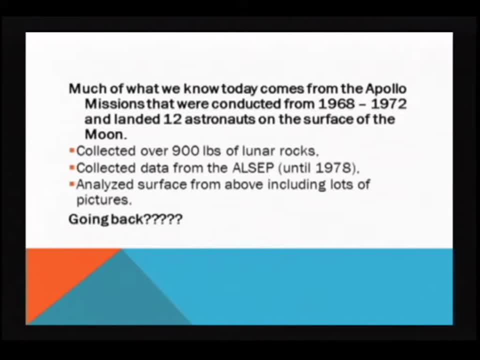 so therefore, we've had six missions that have landed on the moon. One of the things that they did is they collected over 900 pounds of lunar rock so they could physically go ahead and bring those rocks back and it could be studied then in a laboratory here on Earth. 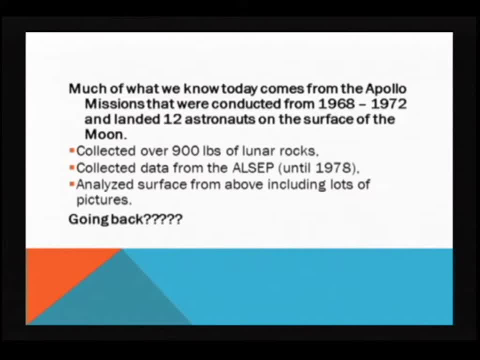 But we find out that of those six missions, only the last one actually had a scientist, a geologist, with them. The rest of them were all astronauts but didn't really have that scientific training. Now all the astronauts did go ahead as they were preparing for the mission. 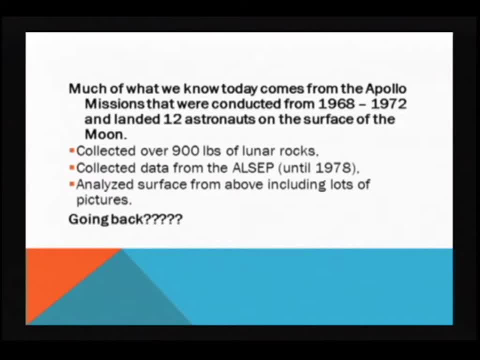 certainly had a lot of geology that they had to learn, But as far as their background they were not actual geologists. Like I said on the Apollo 17,, there was a geologist. They also collected data from a package of scientific instruments. 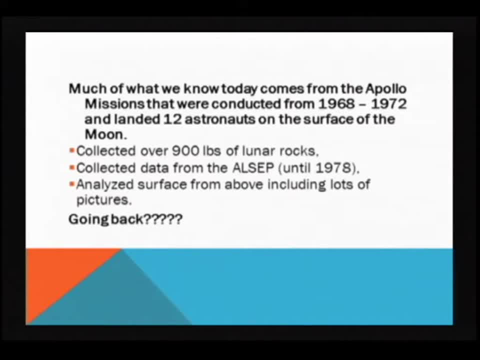 that they left on the moon and that was until about 1978. So notice, that was about six years after the last Apollo mission And they analyzed the surface from above again, including lots and lots and lots of pictures. The other thing that they did 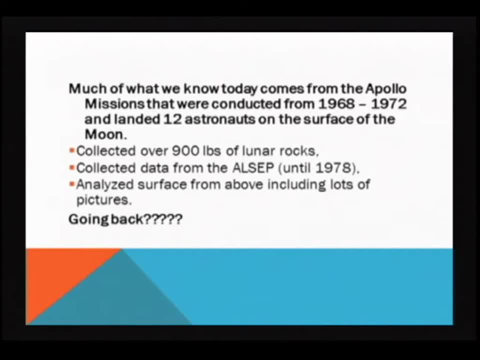 and remember that was one of the first ones where, again, really looking at what was going on was looking at what was going on in space, And so there was a lot of physiological experiments that were occurring to see what mankind was going to be like in a long time in space itself. 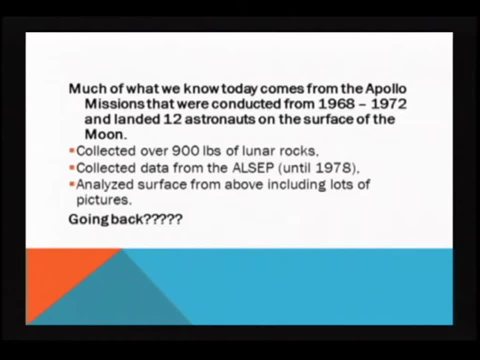 You know, going back, who knows at this point, At one time I think everybody thought we'd probably have some kind of small colony on the moon, Certainly by the 21st century. you know, I think with the way money issues have become and cutbacks and everything else, 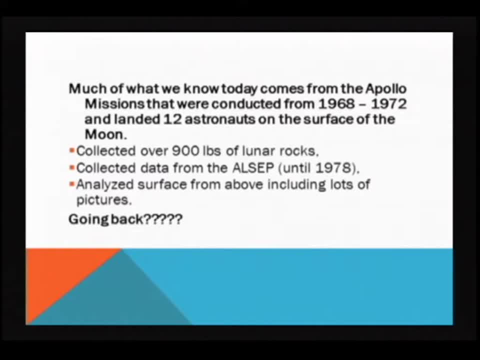 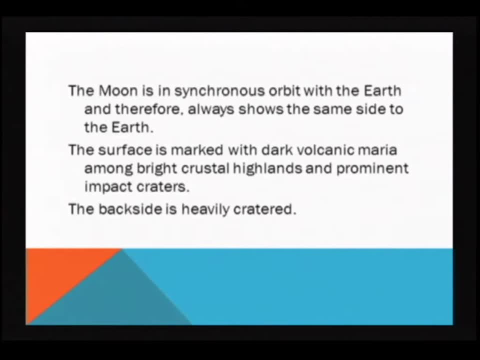 I don't know whether we'll actually go back. My guess- and it's certainly just a guess- is that we might end up going to Mars before we go back to the moon. The moon is in synchronous orbit with the Earth and, if you remember when we talked about the phases of the moon, 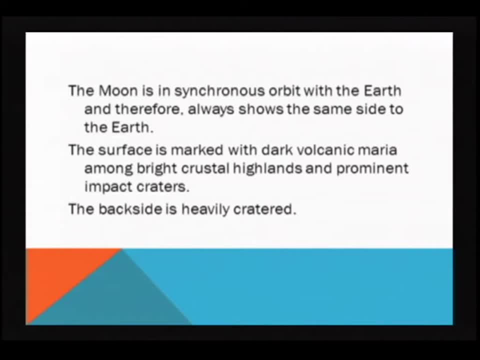 we always keep that one side toward us. Well, that's what we mean in being in locked and synchronous orbit. It's always showing the same side to the Earth. But that means, then, that the amount of time that it takes for the Earth to go around, 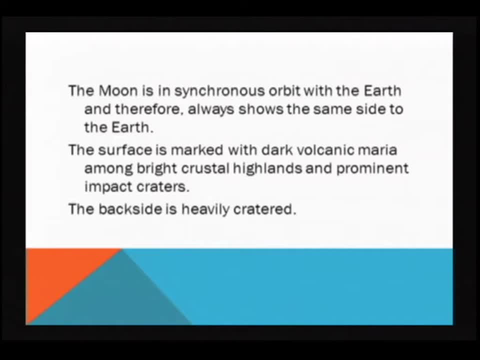 excuse me, for the moon to go around the Earth is exactly the same time as it takes for the moon to go rotate once on its axis And as you've seen pictures of the moon, you know that it's marked with very dark volcanic mirrors. 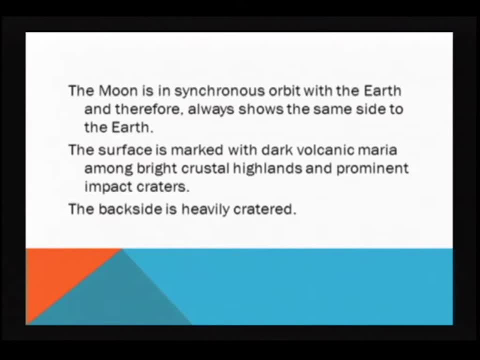 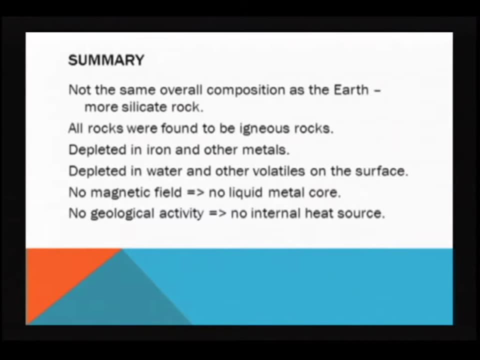 with very bright crustal highlands and then very prominent impact craters And then the back side is extremely heavily cratered. If I look at just kind of a summary of overall what not only the Apollo missions have found but just in general as we have studied the moon, 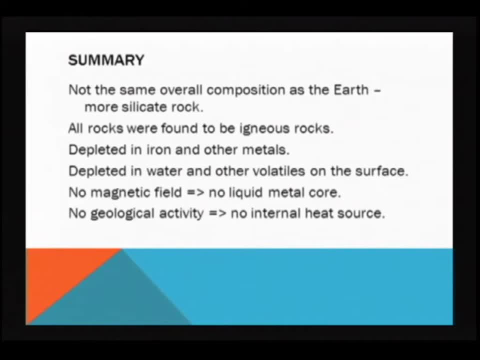 it doesn't seem to be the same overall composition as the Earth. It seems to have more silicate rock. Well, that's going to help give us an indication of you know where the moon came from. There are several hypotheses. Hopefully then we can narrow it down. 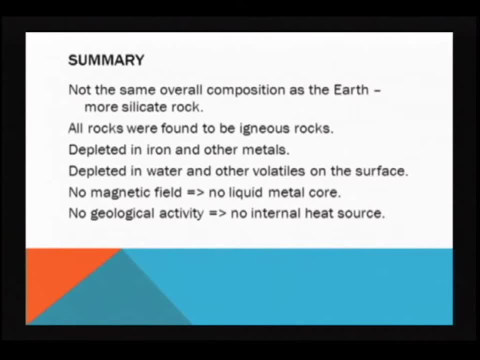 All rocks are found to be igneous rocks. Now think about where we have igneous rocks here on the Earth. You have those where you find volcanism and where you find lava that's gone ahead and solidified, And so that seems to fit with the idea of what we think was going on on the moon. 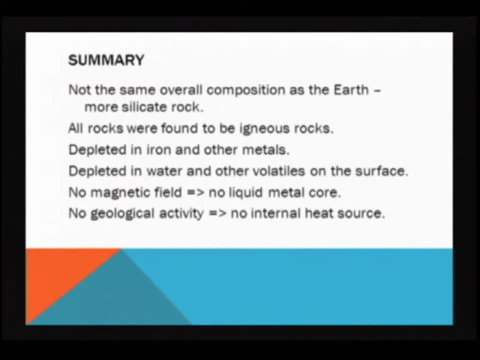 It's depleted in iron and other kind of metals. It's also depleted in water and other volatiles on the surface. Now, I was very careful here to say on the surface, because we do think that there might be water below the surface And there have been some experiments where they have gone ahead. 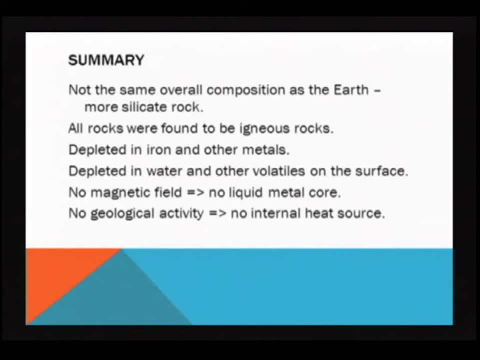 and blasted material off of the moon to look at what was going on below the surface of the moon. And there is some indication. there is certainly water there. There's no magnetic field which tells us right there that there's no liquid metal core. 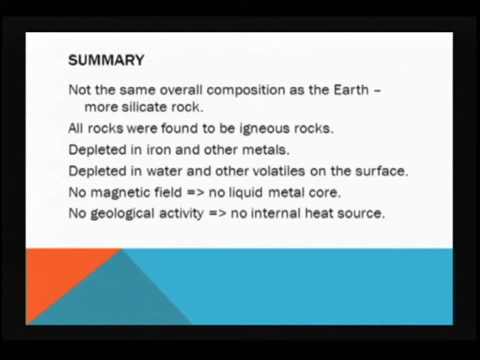 And there's no geological activity. And that's probably because the moon itself is small. It has lost all of its heat And there's no kind of mechanism within the core of the moon to go ahead and produce an internal heat source. So therefore you don't have any kind of geological activity now. 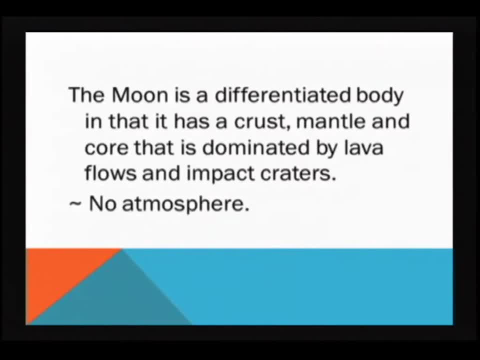 from what's going on within the moon itself. We do know that the moon is a differentiated body, And so that means, guys, remember, it has a crust, it has a mantle and it has a core, But the surface is basically dominated by lava flow and impact craters. 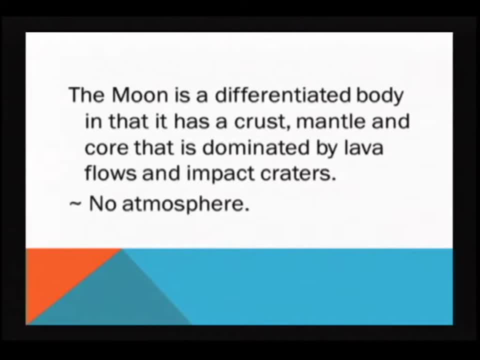 Now we've got to think about, if there's really no internal heat, where is that lava coming from? So we'll talk about that here in just a minute. with those impact craters We also know the moon has essentially no atmosphere. It's simply too small to really go ahead and hold any kind of atmosphere at all. 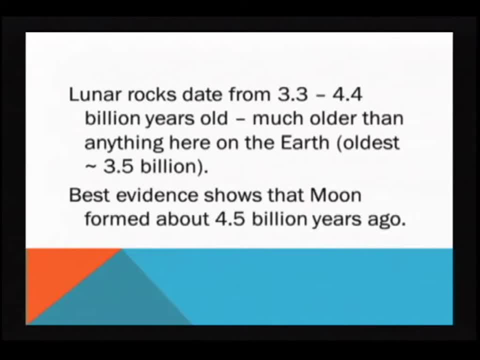 Lunar rocks seem to date from about 3.3 to about 4.4 billion years ago. Now, that's older than anything that we have here on the Earth, because the oldest rocks that we have here on the Earth are 3.5 billion years ago. 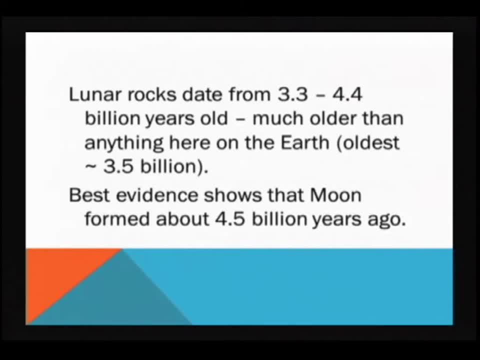 So what's going on? Well, if you think about it, on the Earth we certainly have an atmosphere, We have water, We have wind, We have all the kinds of things that we need to produce weathering and erosion. We also have plate tectonics. 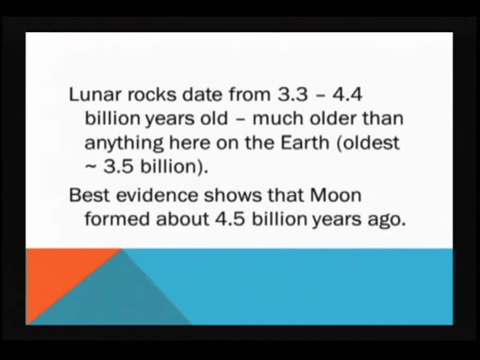 So you have material that is being destroyed. At the same time, you have material that's being produced, And so the fact that on the moon we don't have any weathering and erosion, we don't have any climate to go ahead and cause that. 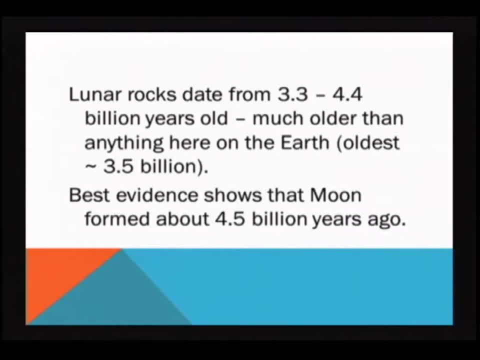 you know, once those rocks were originally formed, they're there, They haven't moved, They haven't changed And they're not going to. There is chemical weathering, but that's more from the sun impacting on the surface itself. So there's a little bit. 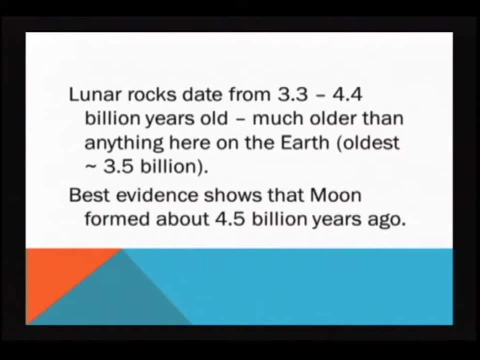 So that's a little bit different, And we do see a lot of dust on the moon which is from that, But as far as any kind of mechanism to really recycle the rocks that we see on the moon, that's not there, And so that's why we do see older rocks on the moon. 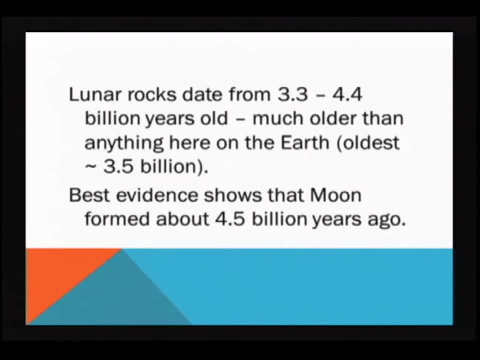 even though we think that the moon and the Earth are about the same age. So best evidence shows that the moon formed about 4.5 billion years ago, which is about when we expected the Earth to have formed, So still formed around the same time. 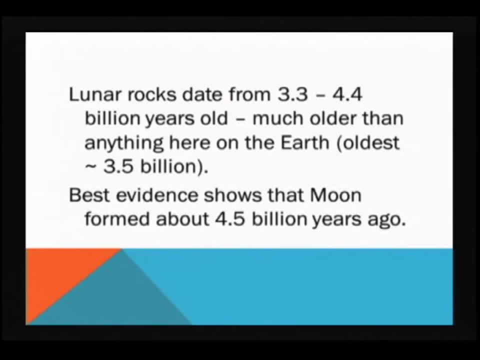 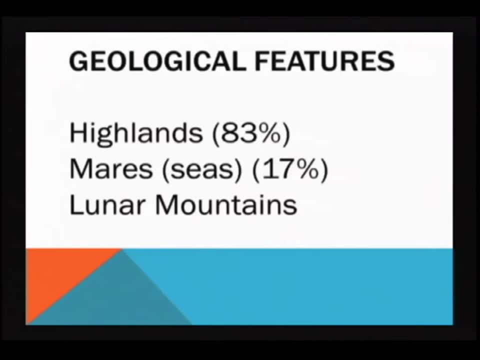 but the rocks that we see on the moon are much older than rocks here on the Earth. Now we have several geological features. We have the highlands, We have the mares or the lowlands, And then we have lunar mountains And, as we've talked about, the planets that we see through our solar system. 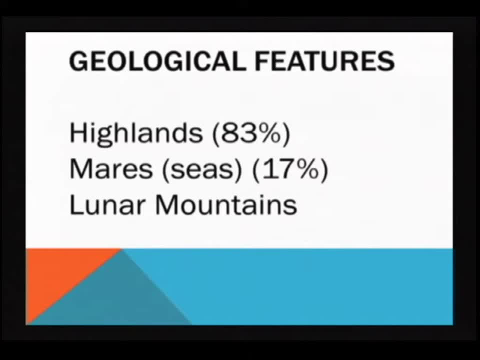 at least the ones that were terrestrial. they all seem to have highlands and lowlands, So it was kind of expected to see those same kinds of things on several of the moons, And you can see percentages there: About 83% of the moon is the highlands. 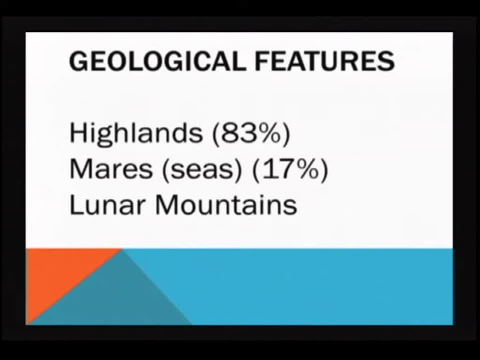 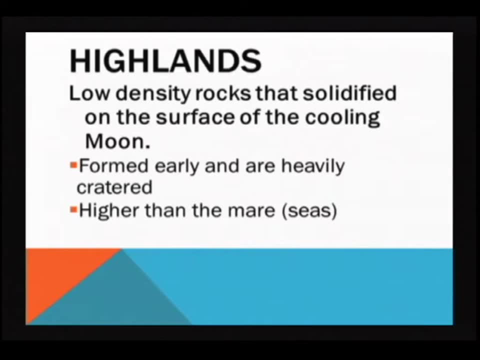 About 17% are those mares or those seas, And then the fact that you have those mountains that are going to be then on the surface itself. So now let's talk about the highlands. Those are low-density rocks that have solidified on the surface of the cooling moon. 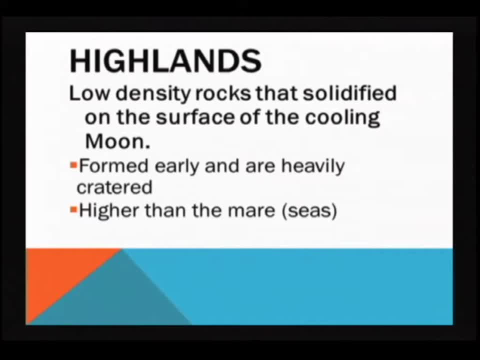 Okay, so let's talk about that lava flow. We know that at one time the moon was very, very warm. I mean, that makes sense. It's in the process of forming you know. So it did go ahead and solidify. 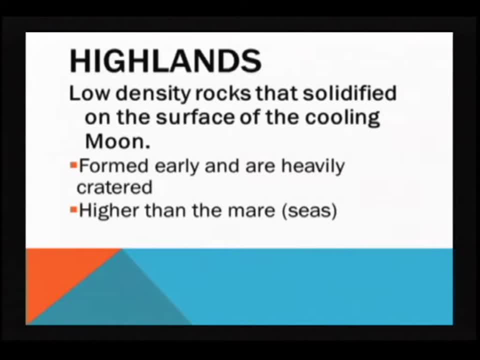 Well, there's where your lava came from. And two, we're going to find that you will have lava flows. when you have something that impacts the surface of the moon, that goes ahead and literally melts where that has impacted, And then that will also go ahead and solidify. 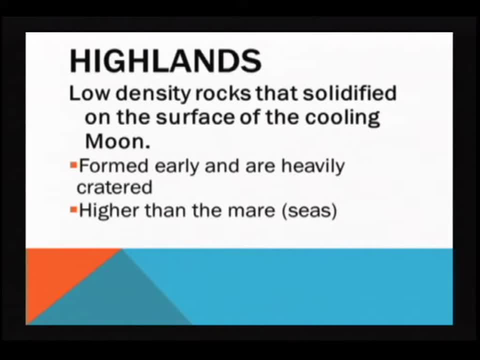 So there's a couple of ways that we can get that lava flowing. It does not have to be from volcanism, which is what we usually see from here on the Earth. I want you to think about the volcanoes and that lava that you see on the Hawaiian mountains or Hawaiian chains. 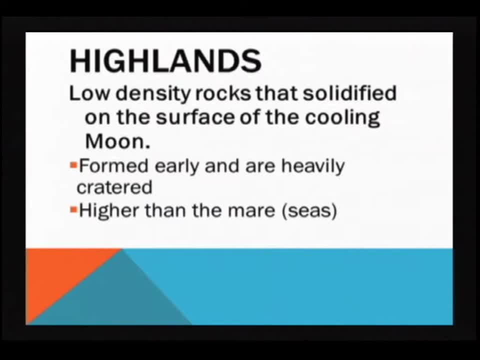 You know, it just kind of oozes up from the ground, And that's the kind of lava flow that we're talking about on the moon. Now, granted, that lava flow is indeed from volcanoes, But if you just think about the fact that something comes in and hits it, 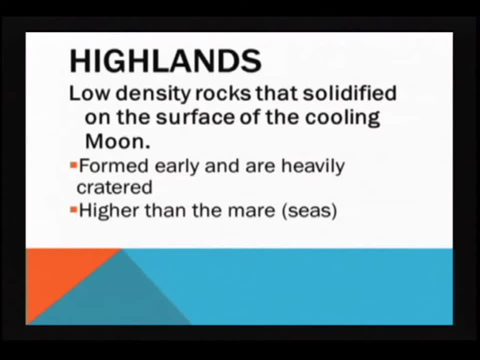 and solidifies that material. it's under a lot of heat at that point And it just kind of oozes up and then goes ahead and flows because it is in the form of a liquid And it'll go ahead then and cool off. 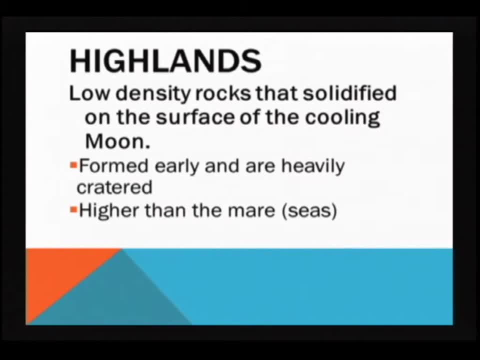 Now the other thing that happens if there were any craters that were already there before. when that lava goes ahead and oozes up and that surface itself has solidified, because of the crater itself, the impact, then you tend to go ahead and cover all of those craters. 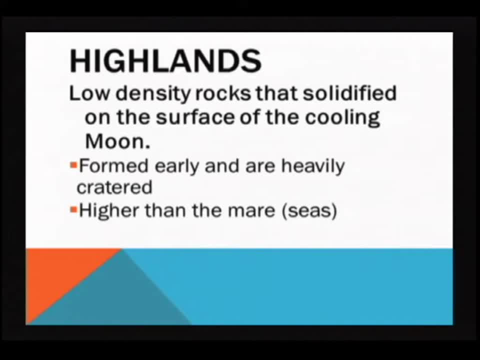 And so they get covered in that then and makes it a little bit more difficult for us to go ahead and actually date the surface of the moon. You may see very few craters because that lava has gone ahead and solidified and basically covered them up. 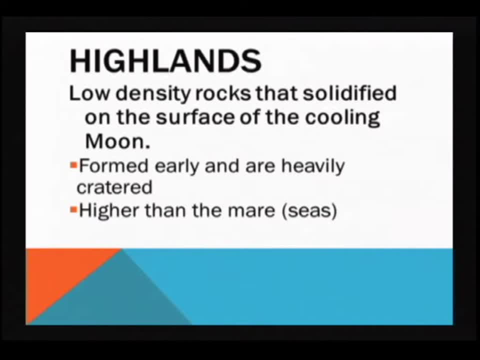 So notice the highlands tend to be formed earlier and heavily cratered. Well, if we know that the lava will go ahead and well up and cover that and we still see lots of craters, we know that that area is extremely old. So remember one of the ways that we can date a surface. 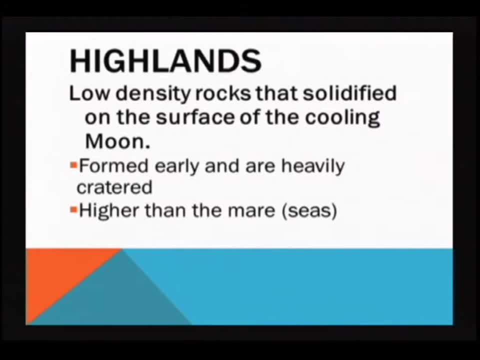 is by looking at the number of craters. We also know, hence the name highland guys, that they are higher than the mares or the seas. Now I need to stress that these are not, in any way, shape or form liquid water. 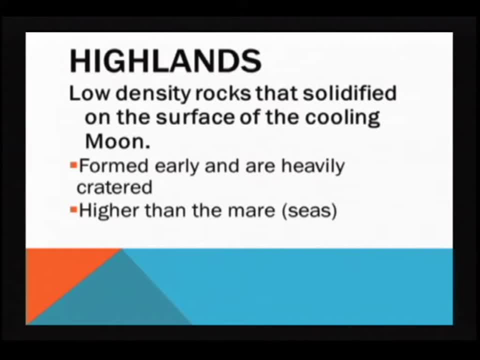 Originally, when ancient people looked up and saw the moon, those dark areas did indeed look like liquid water. But, number one, you don't have an atmosphere, which means even if you had liquid water on the surface, it's going to go ahead and boil off incredibly quickly. 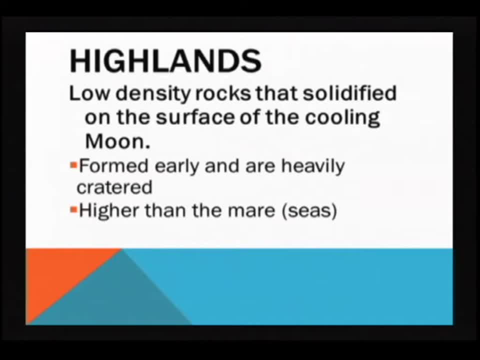 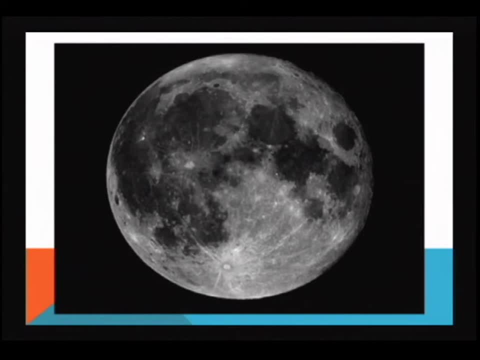 And there's just no way that you're going to have the water on that surface anyway, But we still do. column C's: Now, this is a picture of the front side of the moon, the side that faces us, And I don't know if you've got a really good imagination. 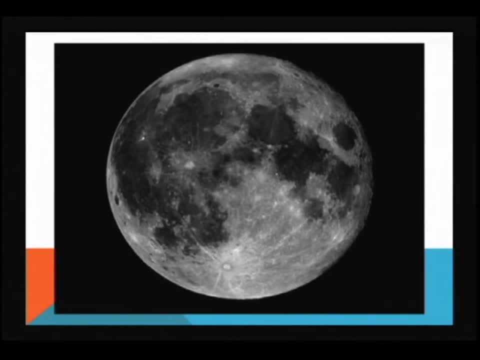 you can go ahead and see the man in the moon there, But it certainly shows those lowlands, those dark areas, those mares or seas, And then you can see that you have in some of those impact craters, and in some of those impact craters you have rays. 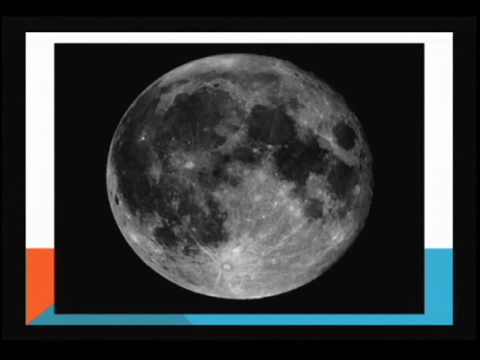 and those rays tend to be very white. Well, we think, then, that that's probably very new material that has not had a chance to undergo the weathering from the sun, And so, given enough time, those rays will eventually become dark, as the sun does go ahead and go through the weathering process. 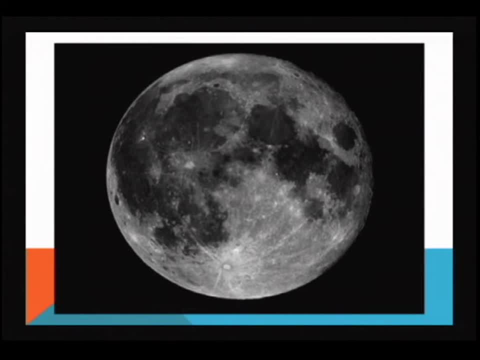 Most of these impact craters that we see- I mean even when we talk about young, you know something that's possibly more than a billion years old. we have seen impact craters that have formed. We've seen on the moon now. 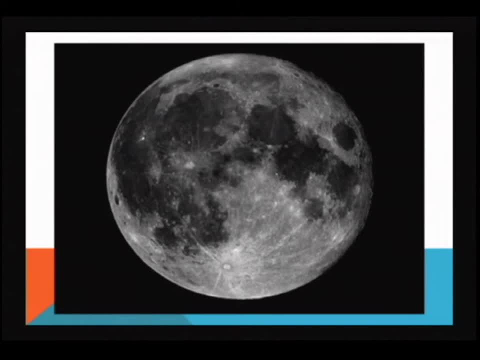 I mean, we see, when you've got the moon in shadow, you can see little light impacts on the surface, and so we think that what happened is something ran into the moon and went ahead and produced in that light as it went ahead and solidified. 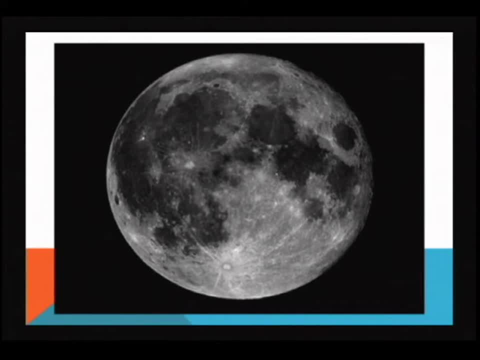 The other thing is we have had in recorded history two monks that were up for breakfast walking across and looked up and saw, and we think, an impact crater on the moon And they've described it as it looked, like the moon was being basically torn in half. 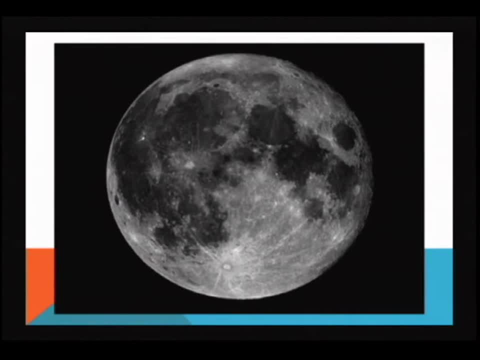 and there were horns that were coming out of it. And so if you look at kind of where they went ahead and said they saw that light, that moon, then there is a relatively new crater on that backside. It is on the backside. 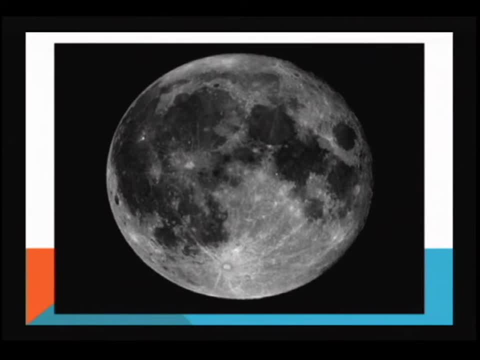 just right on the other side of the part that shows, And so we do think that they probably did indeed see a larger impact on the moon. and then what was left off, as that moon then was going ahead and cooling down. You can't imagine what it would be to kind of look up at the moon. 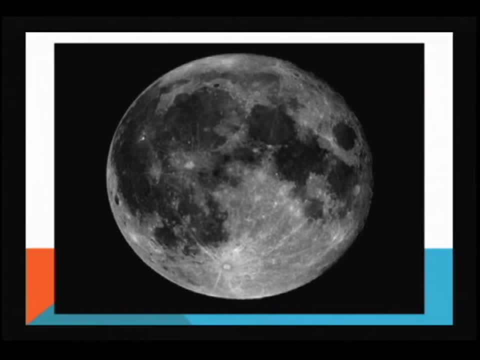 and all of a sudden see an impact crater or see the results of something that hit the moon. But we do have recorded history that they did see that. So again, it's not geologically active from the core itself, but it is certainly active because there's still a lot of things. 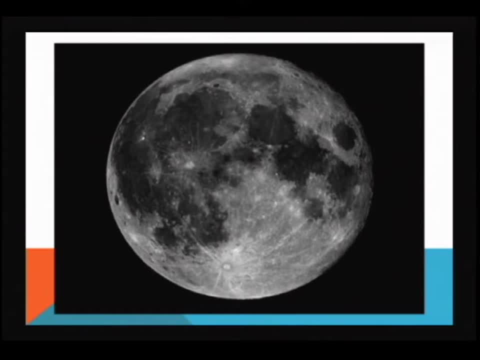 out there in the solar system that are coming by and will tend to run into bodies. I mean, we see that here on Earth all the time with meteorites, fireballs, things like that, The mirrors, those really dark areas right there. 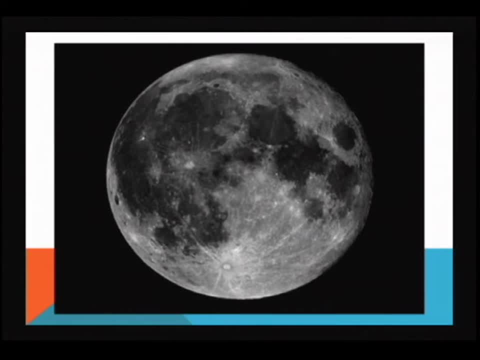 although notice, guys, on this picture, there's one really big impact crater- relatively new, Actually. there's a crater there, There's a couple of them that are sitting in some of those seas, which means, guys, those things happen after the seas formed. 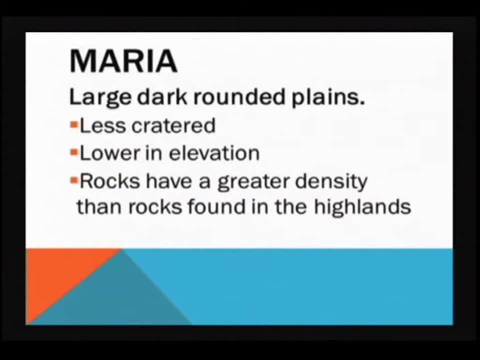 They tend to be very large, dark rounded planes, and we'll see that again in one of the larger moons of Jupiter, actually the largest moon in the solar system, and that's Ganymede. You'll have those same kinds of very old rounded planes. 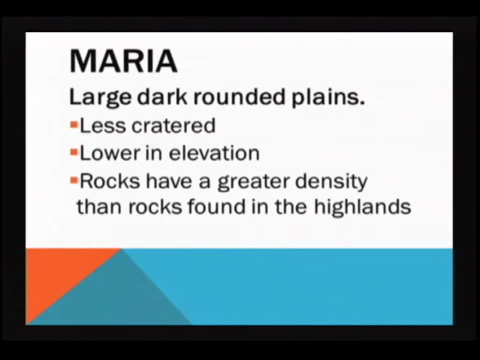 They tend to be less cratered, but again, that would make sense if they had been solidified and that lava then flow- hence the word flow- went ahead and covered up a lot of those craters, So you would expect those mirrors to be less cratered. 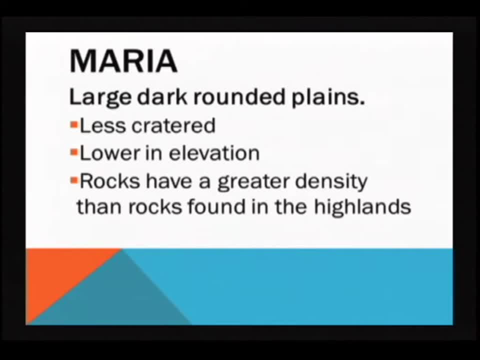 than what was going on with the highlands, Certainly lower in elevation. Think about what happens if we take all the water off the Earth. Then the seas, the bottom of the oceans would certainly be lower at elevation than what the continents are. 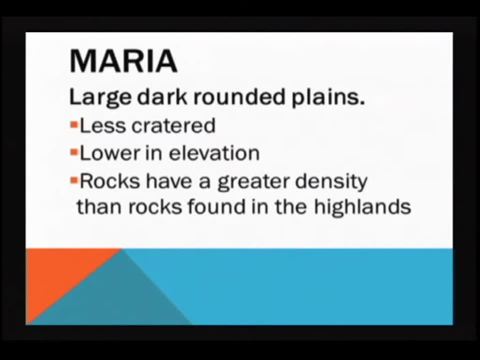 And then we find that the rocks have a higher density than the rocks found in the highlands. So there does seem to be a density in the material relative to where you're going to find it on the moon. Like I said, mirrors are probably impact basins or craters. 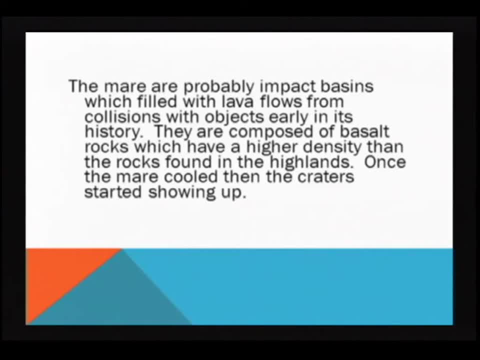 Now we think that early in the solar system- and not just for the moon, but I mean this was throughout the entire solar system- there was a lot of debris that was heading around the solar system, and so we think that about 3.8 billion years ago, 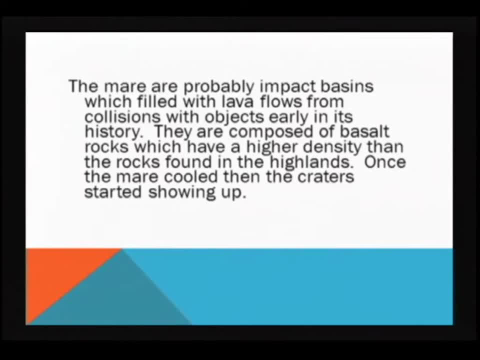 there was a lot more collisions, things like that, as the solar system itself was still in the process of material that was left over and still roaming around, And so you have a lot of those that seem to date back to about 3.8 billion years ago. 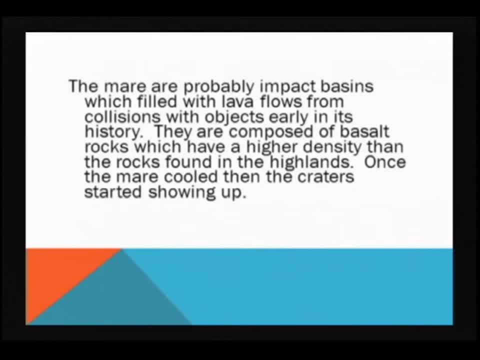 And then it seems like after that time things kind of slowed down. That's about how long it took to go ahead and basically clear out the solar system, all that other material. So then you see that in several things where that seems to have calmed down now, 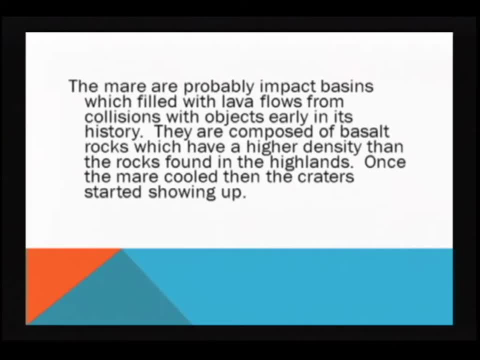 and so we don't quite have quite as much activity in the solar system as we did earlier. So they tend to be composed of basalt rock, basically what our ocean floor is composed of, And once those seas or mares cool, then craters start showing up again. 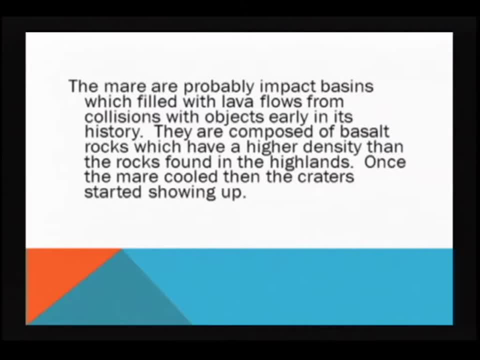 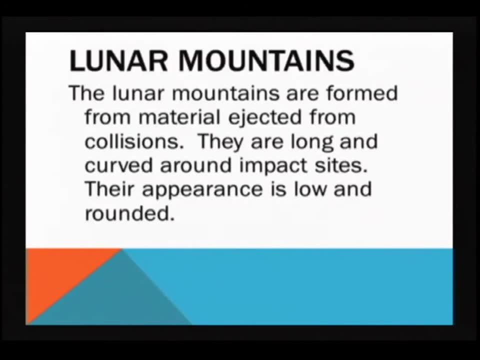 which says that there were still things that were within the solar system moving around, but not nearly to the extent or to the large amount that you had earlier. And then we have lunar mountains, And if you've got, you know, a telescope or something that you're using, 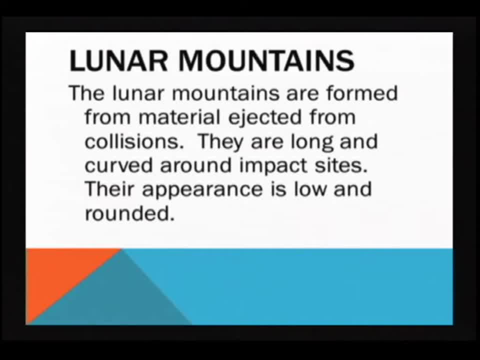 you can actually go up there and observe shadows on the moon as they're being cast from those mountains. So lunar mountains are formed from the material ejected from collisions. They are not formed from plate tectonics. The moon never had plate tectonics. 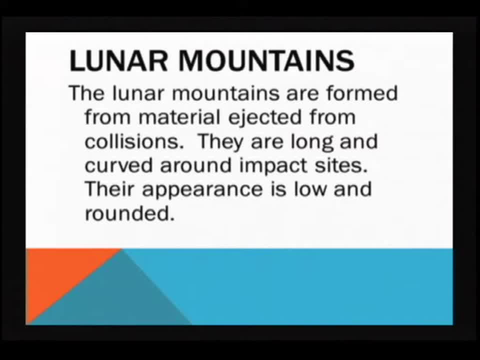 That surface never had enough heat from below to actually go ahead and move around. And so next time you're around a sandbox guys, you know, take a couple of rocks and go toss them in the sand and you'll see that same kind of mechanism. 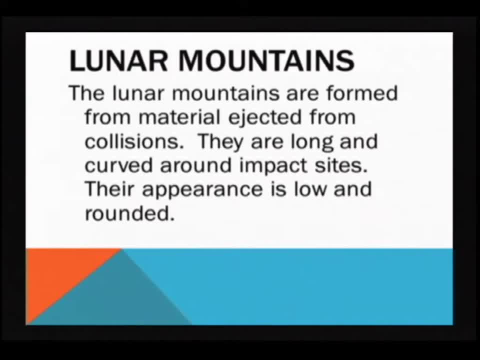 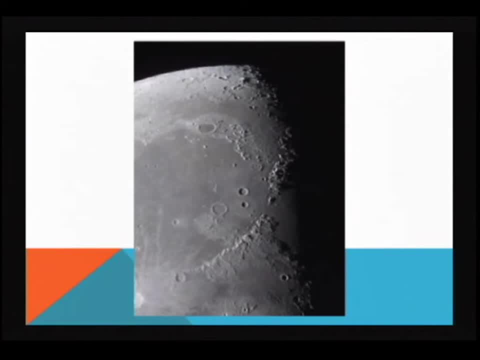 They tend to be very long and curved around the impact sites and their appearance is kind of low and rounded, things like that. And here's a picture of some of those mountains. You can kind of see that a lot of times they ring the impact site. 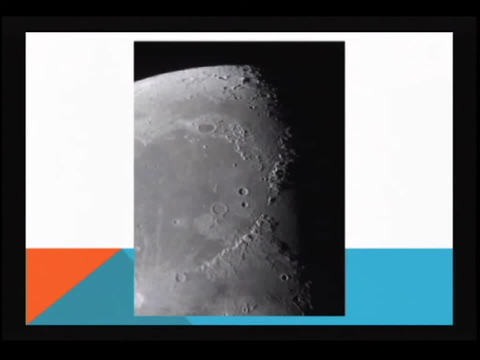 and so they tend to be associated with an impact site, And this also kind of shows you one of the seas and then kind of looks really flat, and then you can see craters that have gone ahead and showed up Very different than what I showed you previously. 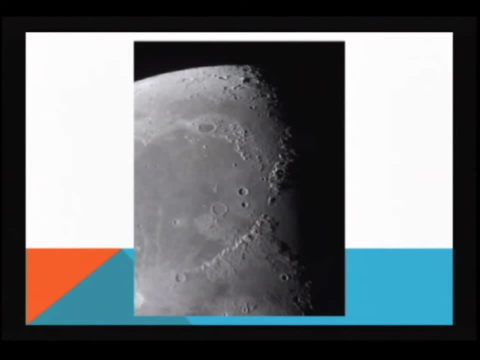 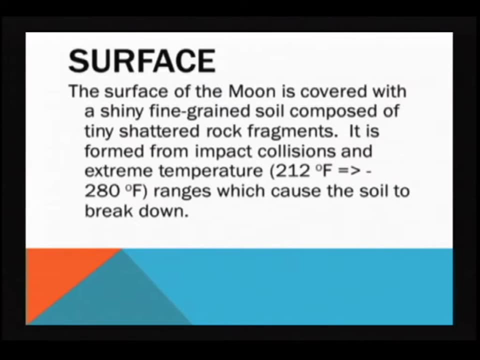 on the back side of the moon and what that looks like Now. the surface of the moon is covered with a really shiny, fine-grained soil and that is composed of tiny, shattered rock fragments. Okay, so how did those tiny rock fragments? I can't say that this morning, guys. 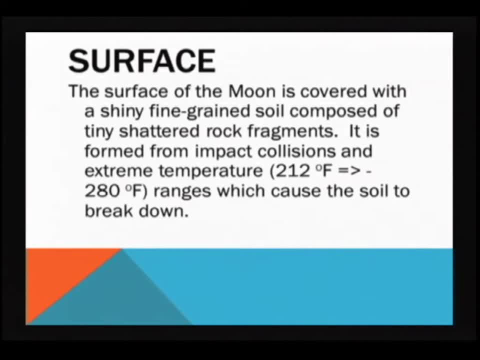 how did those rock fragments actually get shattered? You know there's no wind out there. Well, luckily we've got a way to be able to account for that. A lot of it's from impact collisions and you know, like I said, 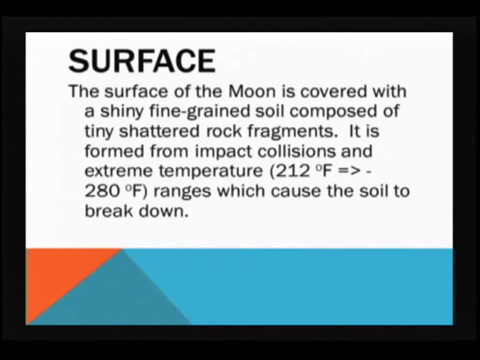 there's still lots of particles roaming around and there's no atmosphere to protect the surface of the moon from. so things come in and you know, even if they're really small, they can go ahead and hit other smaller pieces and break them apart. 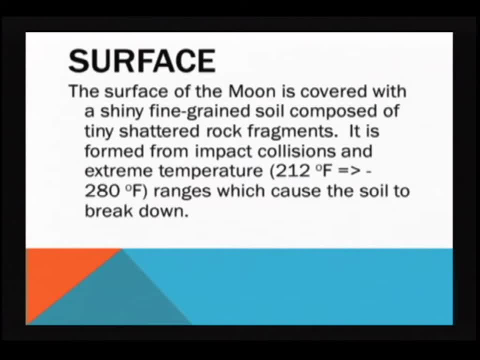 The other thing is you have these extreme temperature ranges. I mean there's no atmosphere on the sun or the moon, so therefore, when it's facing the sun, it's going to get extremely hot. When it's away from the sun, 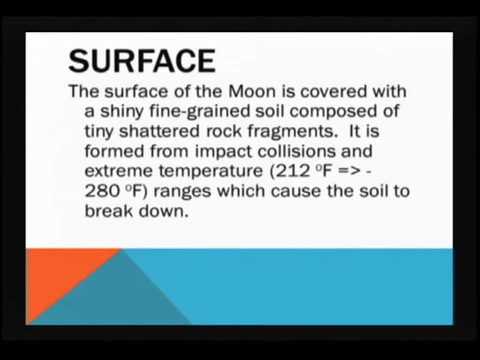 it's going to get extremely cold. Well, think about what your roads look like in the spring, after you've had a winter that's been frozen, and then it's thawed, and frozen and thawed. You have kind of all kinds of pot marks. 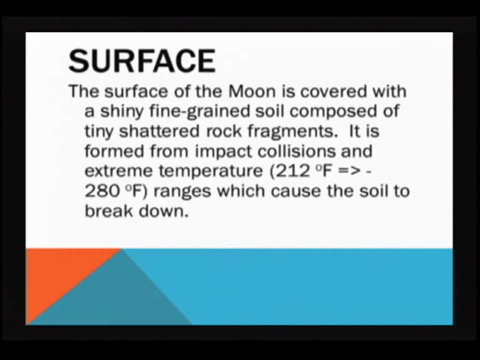 on the roads themselves. Well, that's kind of exactly what's going on here, guys. It's nothing different than the mechanism we see on the Earth, It's just not quite the same range. The Earth is a much smaller range. I mean, imagine, guys, you're almost going. 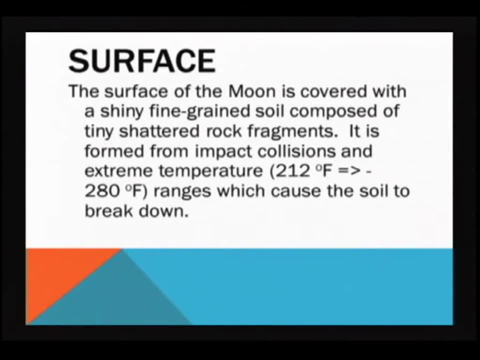 almost 500 degrees difference between the front side and the back side, And so you're going to get that expansion and compression, which is certainly going to go ahead and break down the soil fragments. And so we weren't sure when we first landed on the moon. 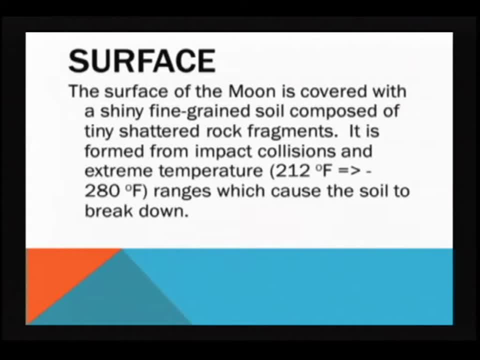 when Apollo 11 went there, whether when it went ahead and landed on the moon, if it was going to sink a great deal into the surface, into that kind of grainy material, or whether the surface itself would go ahead and support it. 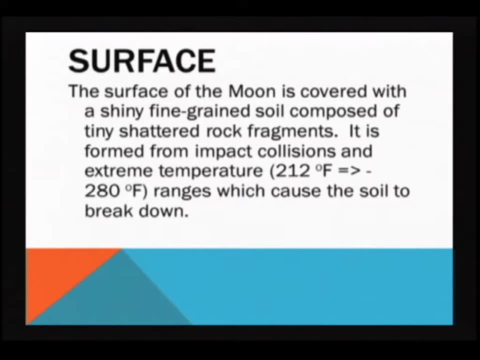 And you probably don't remember, but the legs of the lander, the lunar lander, the bottom of the legs had a very large disk on them, And so that was able then to go ahead and spread that weight out a little bit. 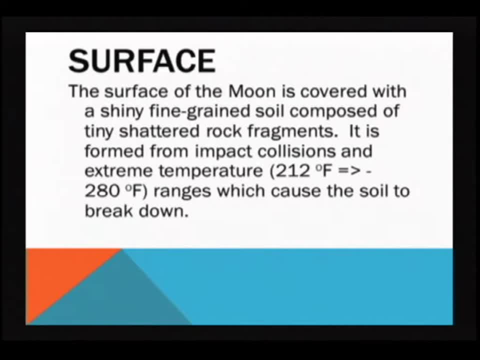 And so if you were going to go ahead and sink a little bit, that disk shape at the end of the legs did go ahead and help support it a little bit. As it turned out that didn't happen, But some people thought that we would sink. 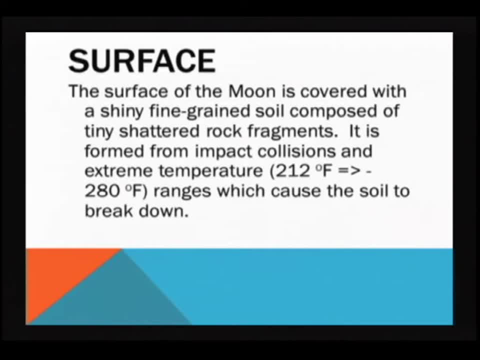 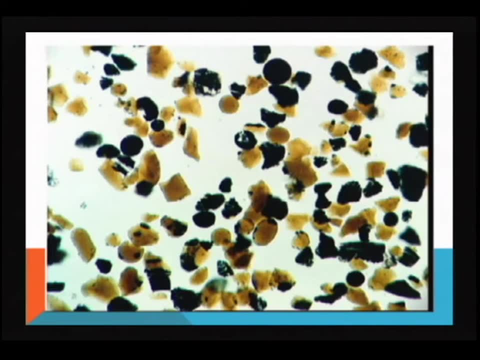 maybe a foot, maybe two feet in all that dust that accumulated on the surface. Now, this is just a picture of the fine grains that you see when you pick up the dust on the moon and go ahead and look at it through a magnifying lens. 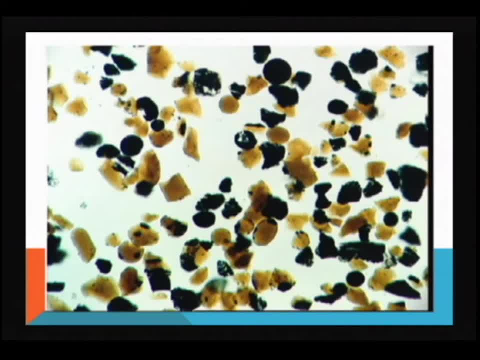 or through a microscope. This is what you see, And if you look at the colors, you'll get some kind of beiges, some blacks. Remember, every time we went to the moon, we certainly picked up lots of moon rocks and brought them back for a total of about 900 pounds. 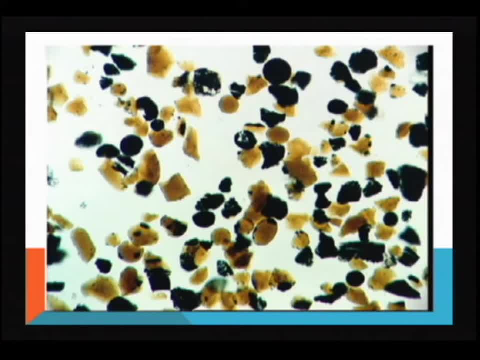 If you guys are ever at the Air and Space Museum in Washington DC, if you go in there, they've got right as you walk in, they've got a big display that has a moon rock and it's in plastic. 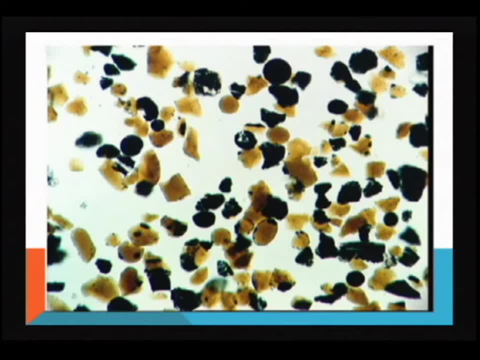 with the exception of the very center, and there's a little plastic disc that's been removed and so you can actually touch one of those moon rocks. And yes, I've been there and I've touched it And it does give you kind of a different feel. 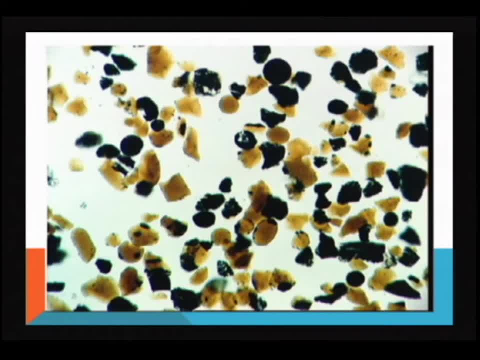 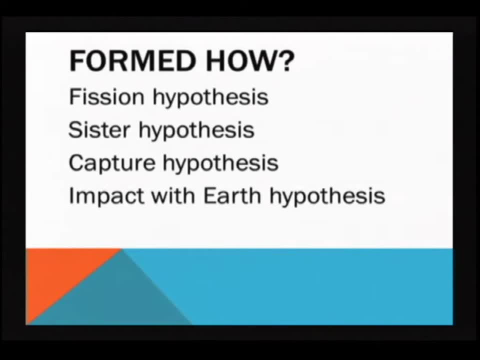 knowing that that's not a rock that's here on the Earth, that that's a rock that came from the moon. So then the question becomes: how did the moon form? And that's really going to be a question for all of the moons. 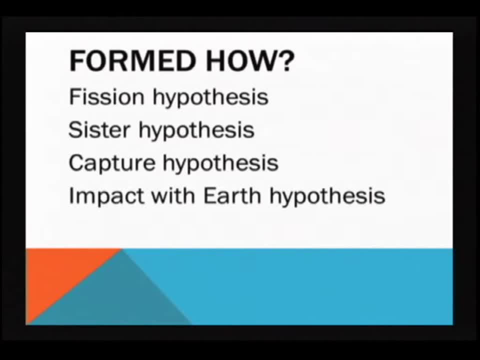 We generally are going to have really big moons, and those big moons tend to be very symmetrical, tend to be very round. Then we have really small irregular moons. Well, we think the irregular moons are basically captured asteroids, which we'll talk about the next time. 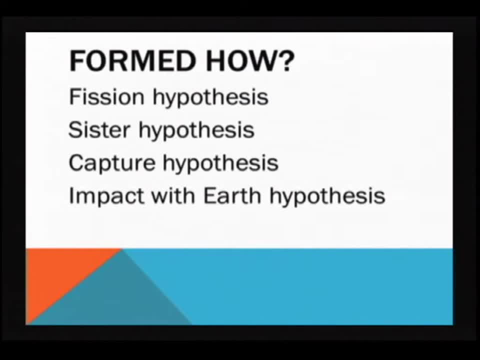 But how did those really regular moons form? Well, if we're thinking about the Earth and our moon system, there's four hypotheses. There's a fission, the sister hypothesis, the captured hypothesis and then the impact with the Earth hypothesis. 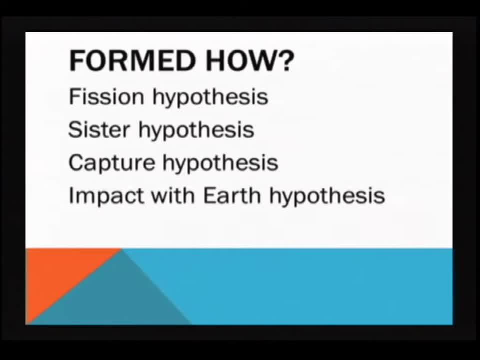 The fission hypothesis just says that when the Earth was originally forming, that it actually split and it formed the moon and the Earth right at the same time, So that basically, you have a cell, that cell splits, we have the moon and we have the Earth. 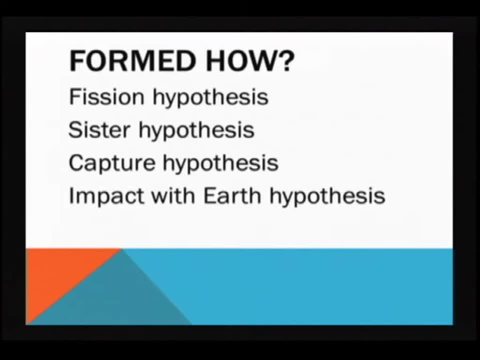 Then we have the sister hypothesis that said, no, that what happened is the moon and the Earth formed at the same time, right beside each other. And then we have that capture hypothesis that says, okay, we have the Earth here. remember, in the early part of the solar system. 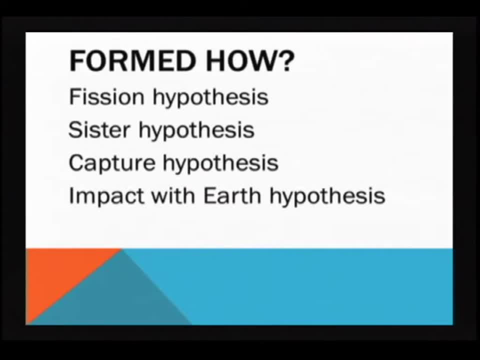 there were lots of things that were roaming around- really big size objects- and that one of those objects got close enough to the Earth to be captured by it And therefore the moon settled down and orbited around the Earth. And then the impact with the Earth hypothesis says. 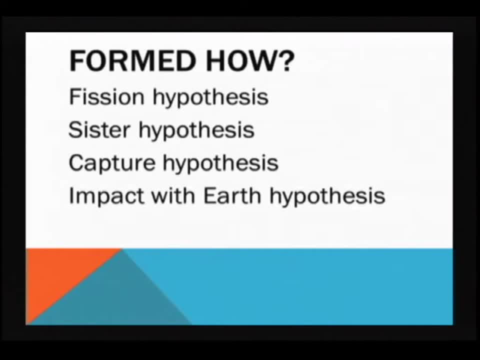 okay, what happened is you had one of these really big objects roaming around in the beginnings of the solar system and it hit the Earth and material from the Earth was ejected, and that ejected material went ahead and formed the moon Now, of those four, 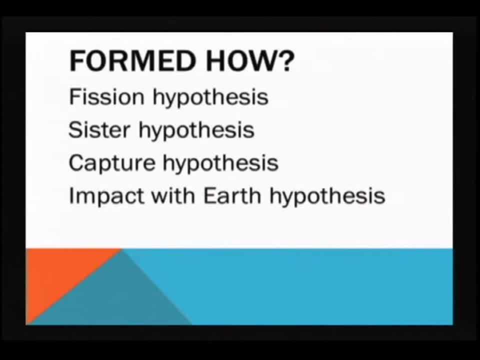 right now the best evidence based on what we found on the moon itself, the composition of the moon- we think that was probably an impact with the Earth. If we look at some of the others- the fission or the sister- that tends to say that you're almost going to have. 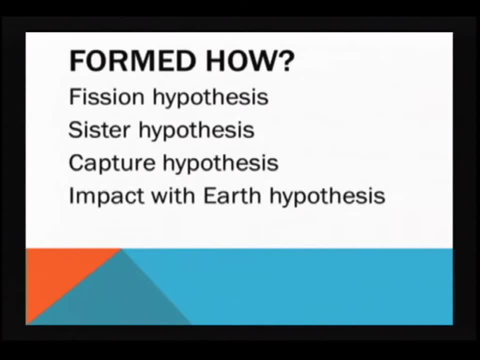 the same type of material, exactly like what you have on the Earth compared to what you have on the moon. But we don't really see that There does seem to be a difference of the material that we have on the moon compared to the Earth. 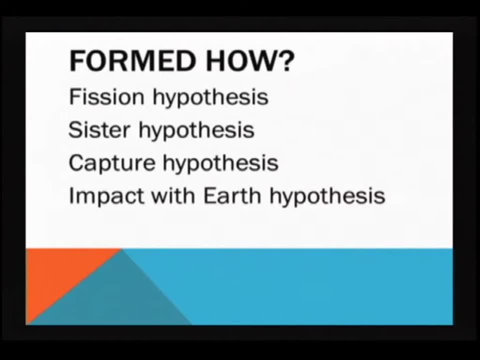 and one of them is the fact that we don't see those iron material or those other metals that we see here on the Earth. Well, if you think about it and that came through and that hit the Earth, you're basically only going to hit the crust. 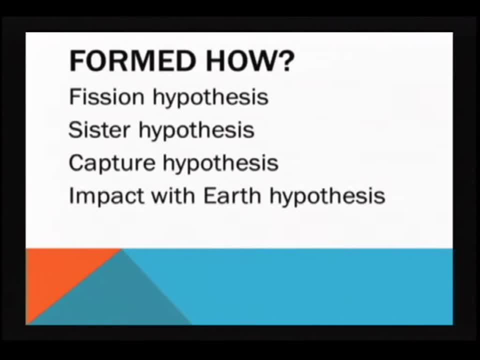 And so the crust is the part that then was ejected and formed the moon. And yes, if we look at the moon and look at its composition, compared with the composition we see of the Earth's crust, then it's a whole lot closer. And so that, as well as some of the characteristics, 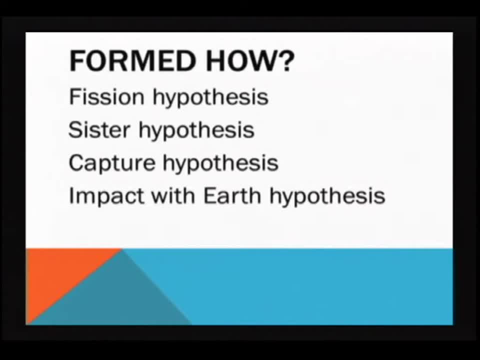 of the moon and how it's related to the Earth with its orbit. we think that that's, right now, the best idea that we have. Do we know exactly? No, We have to just go ahead and look at these, based on the best evidence we have. 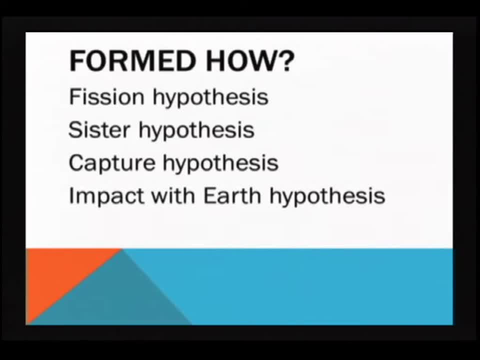 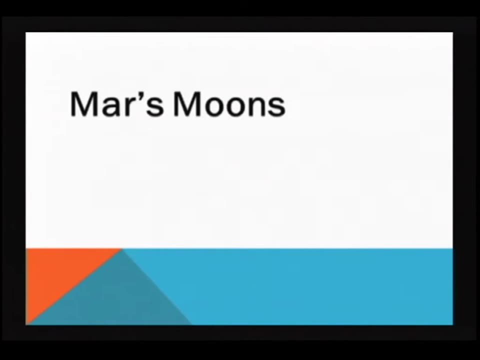 And so it seems like it's probably an impact with something, And we've certainly seen those impacts with Venus, We saw it with Mercury, So we know that those kinds of things existed in the early parts of the solar system. So now Earth has one moon. That's called our moon. Well, let's start backing out and look at the other planets and look at some of their major moons Or, in Mars' case, the only moons that Mars has. Now. Mars has two moons called Phobos and Deimos. 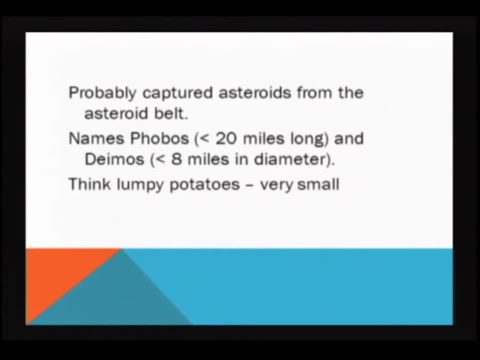 Now remember what our moon looks like. It's this very nice symmetrical round object. Please realize that, guys. when we talk about Phobos and Deimos, we are not talking about anything that remotely resembles anything. that's a nice round shape. 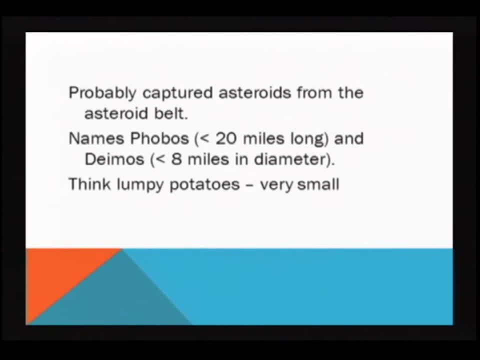 In fact you know, Phobos is less than 20 miles long and Deimos is less than 8 miles in diameter. I mean, if you got a really good head of steam and you went running down Deimos, you probably wouldn't have any trouble running off it. 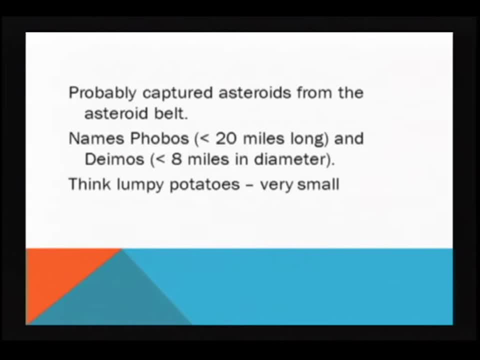 I mean, they are very small And in fact I like to think of them as very small lumpy potatoes. Okay, so where do these lumpy potatoes come from? Well, probably came from captured asteroids. Like I said, remember the asteroid belt. 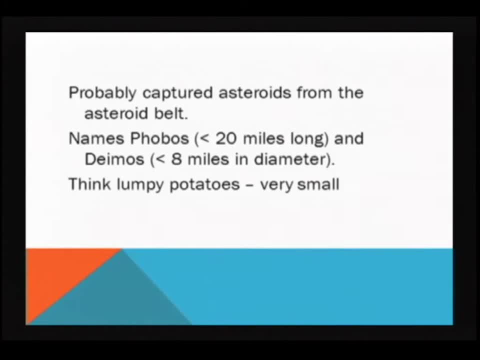 is just right on the other side of Mars, between Mars and Jupiter, And so it's not unheard of to think about the fact that these asteroids could have somehow gotten kicked out of their orbit, headed in toward the inner parts of the solar system. 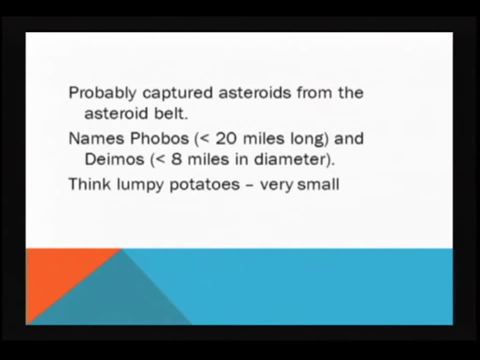 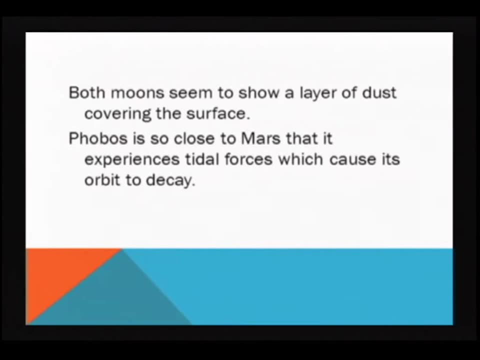 and certainly got close enough to Mars to go ahead and have Mars capture them. Both moons seem to show a layer of dust. Okay, now wait a minute. Let's think about this. We know the moon shows a layer of dust, but the moon is big enough. 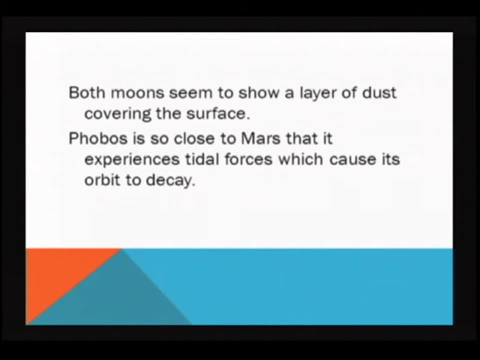 and has enough gravity to go ahead and keep that soil gravitationally bound to it. You know, I mean, if we look at Phobos and Deimos, they're not really very large at all. And so one of the questions becomes: 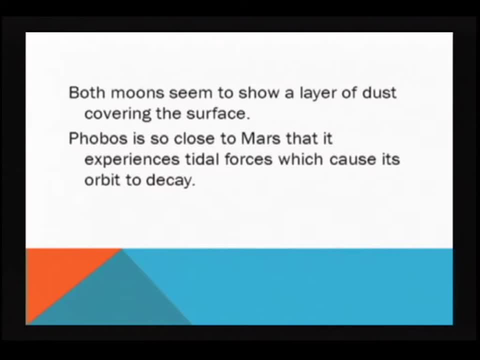 how are they able to keep this dust covering the surface? Why doesn't it kind of leak off? Well, there might be several reasons that doesn't happen. One of them might be close enough to the, or they're far enough from the sun. 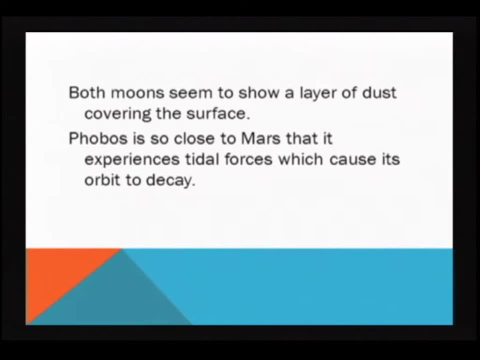 that you don't have a lot of heating there, so therefore there's simply not enough energy to go ahead and kick them off, But still it's kind of surprising that they have that layer of dust. Also Phobos, which is the one that's closest to Mars. 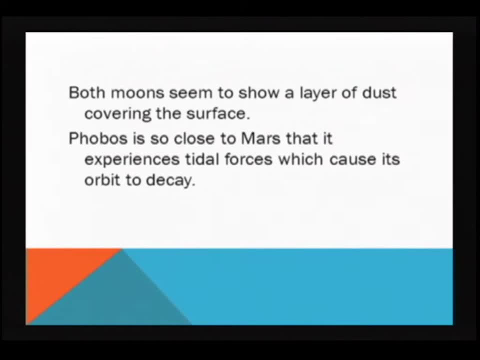 experiences tidal forces from Mars because it is so close And if you look at Phobos's orbit, it is in the process of decaying, which means you know eventually, some point in the future. you know several million years. 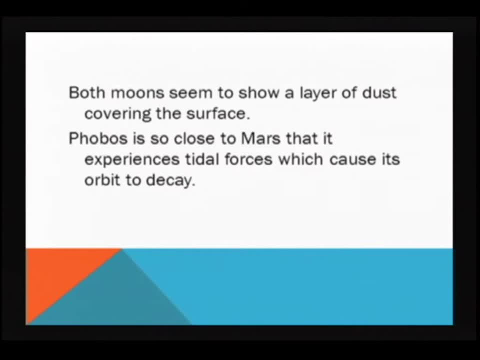 Phobos will probably run into Mars. It's not going to survive. It's simply too close, and Mars is pulling on it all the time. It's tugging on it, And so it'll eventually hit the surface Or, as it comes down. 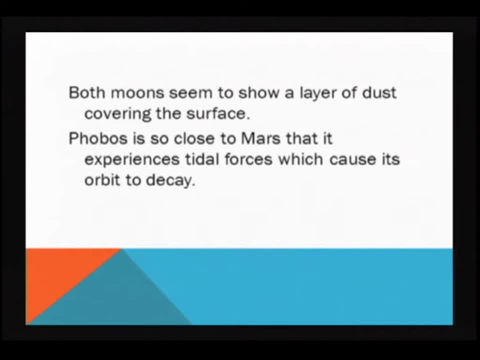 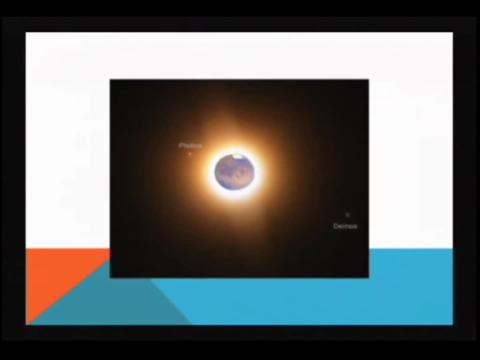 it could be ejected, you know, depending on how much speed it still has when it comes down, but it's not going to remain forever around Mars. So this is a picture of Mars showing you Phobos and Deimos And, like I said, Phobos is certainly the one that's closest. 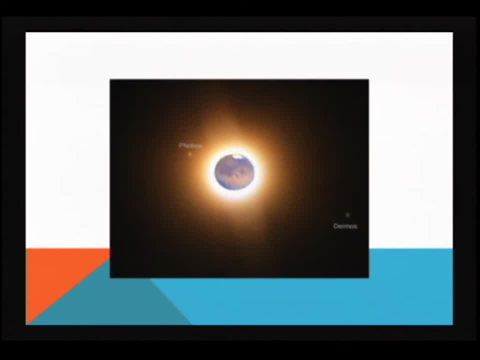 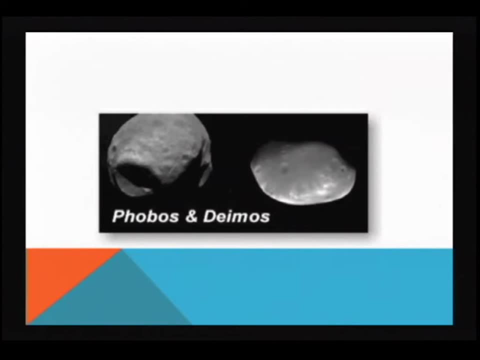 You can see that Deimos is all the way out a little bit further out, And let me show you what those two look like in comparison. There's Phobos and there's Deimos. So you know, they're certainly not. 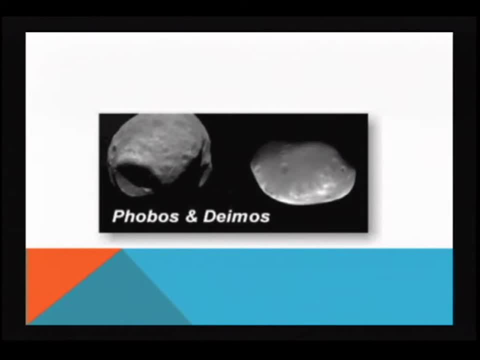 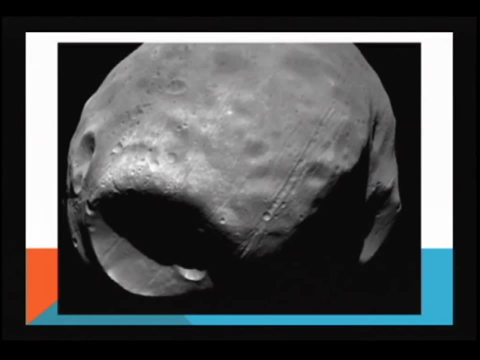 looking like our moon And Phobos and actually, to some extent, Deimos, certainly shows impact craters. I mean, look at that impact crater on Phobos. I mean that was a pretty good-sized impact crater. Coming from the asteroid belt, you know you would expect those asteroids to run into each other, things like that, And you can see there's other impact craters on Phobos Also notice that there seems to be very long kind of straight lines or striations. 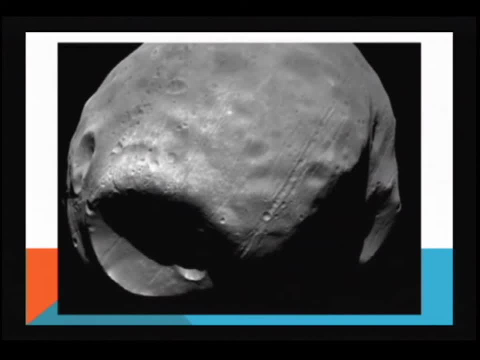 That seem to move backwards from that crater itself And looking at it, you can certainly see that, as I said, there are other impact craters. In fact, there's an impact crater in the big crater that's on Phobos. 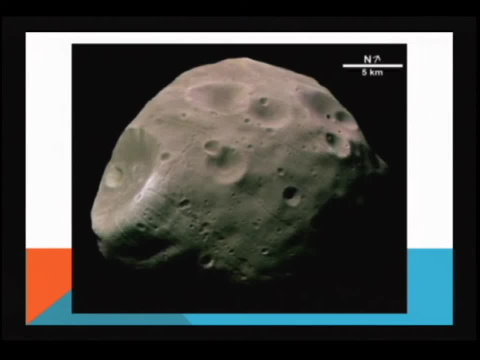 And then Deimos also looks like it has been hit and had material ejected off of it, as well as some others. And then you see they're kind of rounded and in some cases look like they hit at an angle. In some cases you can see a very nice crater there. 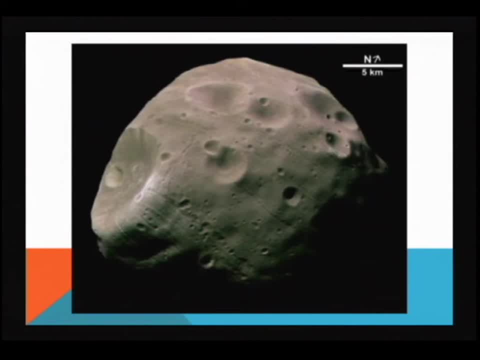 that does indeed have some depth on it. Some of them are very shallow Again, not very large. You get a really good game of basketball on there, or baseball and man. you hit that baseball with that bat and I mean you're not going to find that baseball anymore. It's going to take off. So, captured asteroids, certainly very different than what our Moon is like, And then, as we go on to Jupiter and beyond, you're going to find that Jupiter and Saturn, Uranus and Neptune have moons like the Earth. 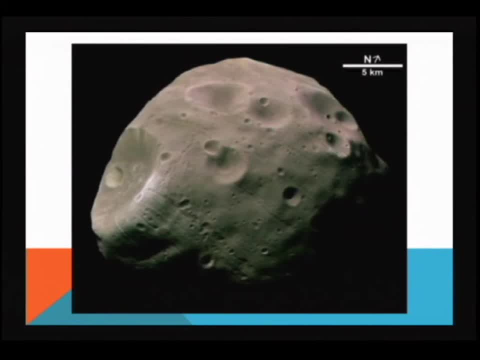 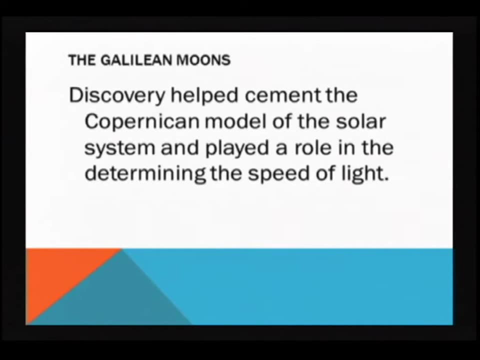 but then they also have a lot of moons like the ones around Mars. So let's go ahead and talk about Jupiter's moons. Jupiter has four main moons, and those are called the Galilean moons. Galileo discovered them, Remember. we kind of talked about that. 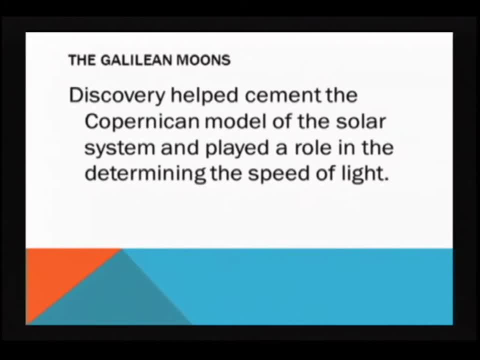 in the first part, when we talked about what happens with the idea that you have the Sun. It's at the center of the solar system as opposed to the Earth. So that was called a heliocentric model and that was proposed by Copernicus. 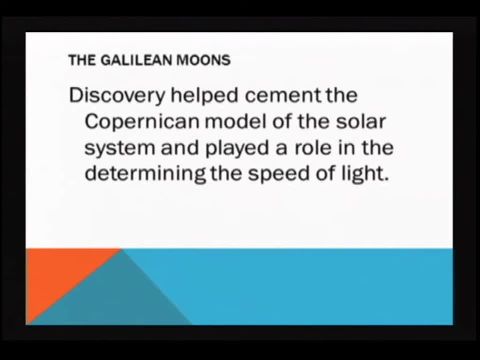 Well, when Galileo looked at Jupiter, it was very obvious that there were four moons that were very bright and you could see them going around Jupiter, And so that meant that, yeah, not everything then went around the Earth, And so that kind of helped seal the idea that 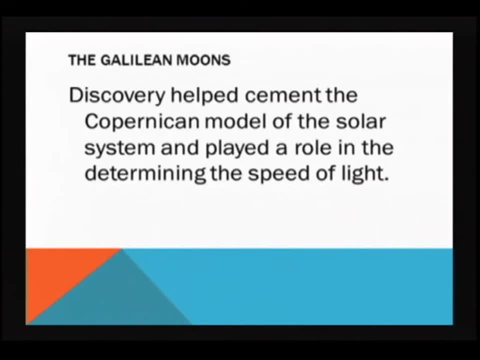 yes, the Sun was at the center of the solar system. You had our moon going around us. You had the Galilean moons going around Jupiter And any other moons that you might have out there were going around the individual planets. The other thing is they played a role. 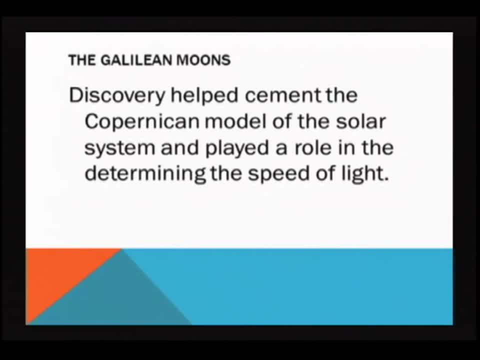 in determining the speed of light. And they did that because we were looking at predicting exactly when those moons would come out from behind the planet, in this case from Jupiter, And when they would do that and they would actually go ahead and measure it. 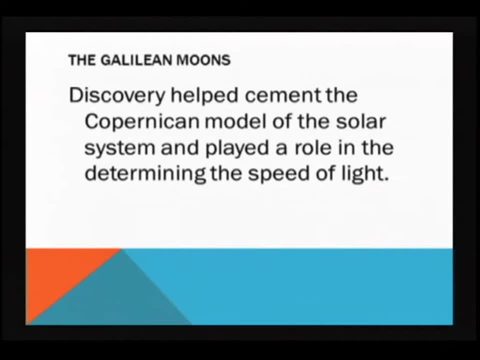 their predictions were always off just a little bit- not much, but just a little bit- And what they realized is that they were. the reason that timing was off a little bit was because of the time that it took the light to go from Jupiter all the way to the Earth. 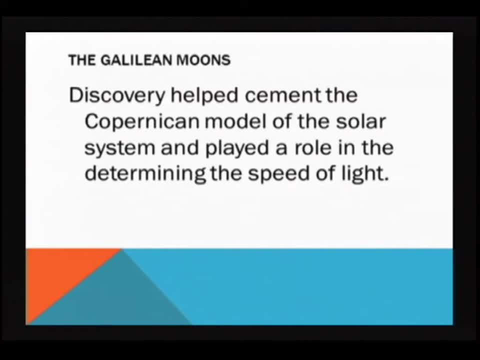 And so they were able then, once they knew that distance from Jupiter to the Earth, to go ahead and determine what the speed of light was. As you know, the speed of light's 3 times 10 to the 8th meters per second. 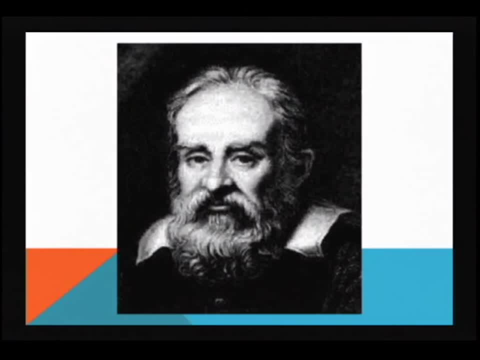 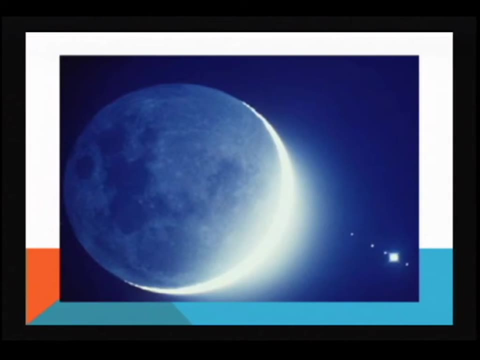 or 186,000 miles per second. This is Galileo, just because of the Galilean moons, So he's given credit with discovering them. Here you have the moon, and then you have the four moons, Galilean moons, of Jupiter, then 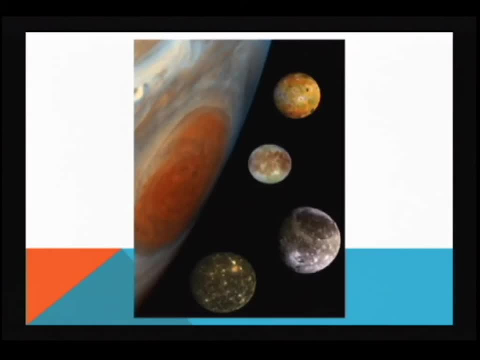 down in the lower right. Here's another picture of them with Jupiter. Now, guys, that's not where they are relative to Jupiter, but putting Jupiter and then putting the moon and the four moons beside it. So we have Io, we have Europa. 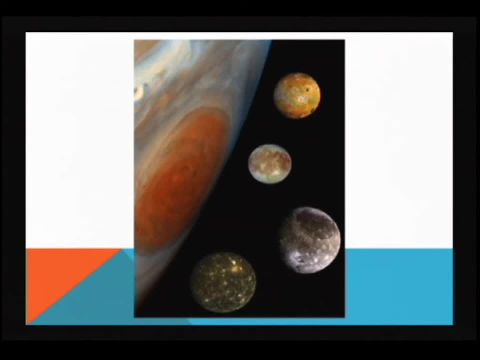 we have Ganymede and we have Callisto, Io being the one at the top, and then Europa, Ganymede being the one a little bit to the right and that is the largest moon in the solar system, And then Callisto being the one down at the bottom. 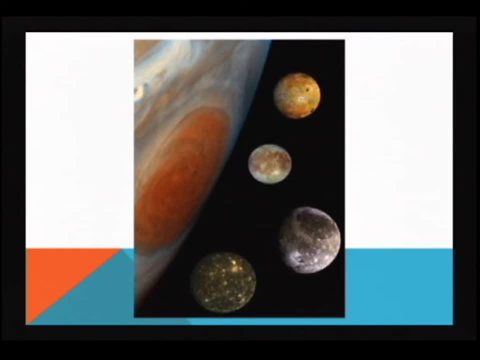 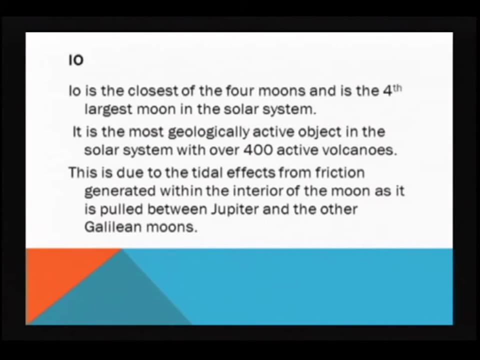 And all four of them are extremely different characteristics. So let's go ahead and start talking about Io, which is the closest of the four moons, And it's the fourth largest moon in the solar system. And, guys, it is the most geologically active object. 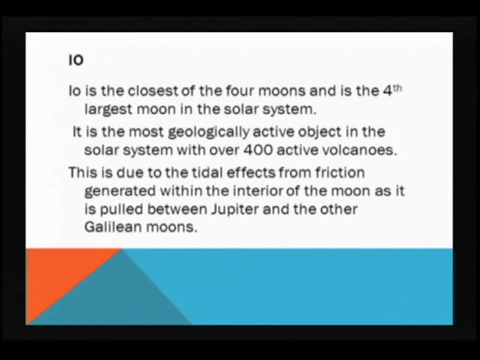 in the solar system, and that includes any of the planets or anything else. You've got this moon that has over 400 active- and I do stress the word active- volcanoes. I mean guys, that's some of the youngest real estate. 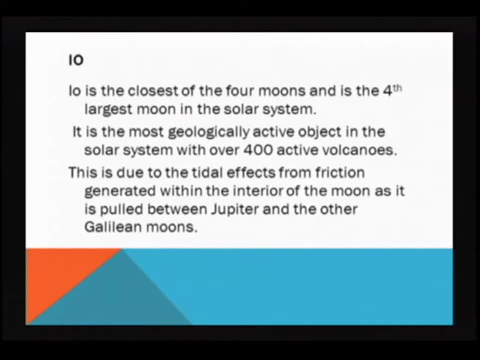 in the solar system. So now, how are we getting that moon to be so geologically active? Why does it have all these volcanoes? What's going on with the core of Io that it is continually spewing material out? Well, guys, I want you to think about. 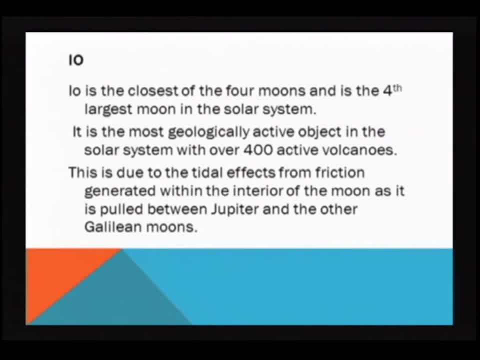 a nice, beautiful, sunny day and you've gone to the fair And you know fair food. you know you've got all those. you know corn dogs, you've got cotton candy, you have funnel cakes, you have Dr Peppers. 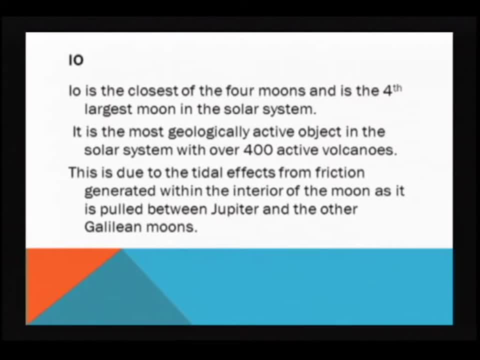 you know you have all of this stuff And I want you to think about, well, what would happen if you ate every bit of that, every bit of that that you possibly could. So you've been at the fair for a good eight or nine hours. 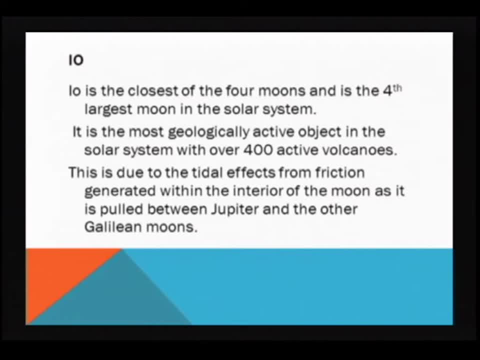 and you have eaten everything you could possibly eat. And then you decide, hey, what I'm going to do is I'm going to get on the tilt-a-whirl, or I'm going to get on the octopus, or I'm going to get on one of these roller coasters. 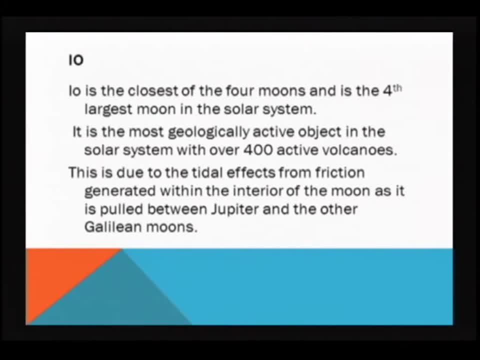 I'm going to get on something that's going to spin me like crazy and drop the bottom of the floor out. Okay, So you do that all within about 30 minutes. You've had all this food. you get on all these crazy rides that spins you and pushes you. 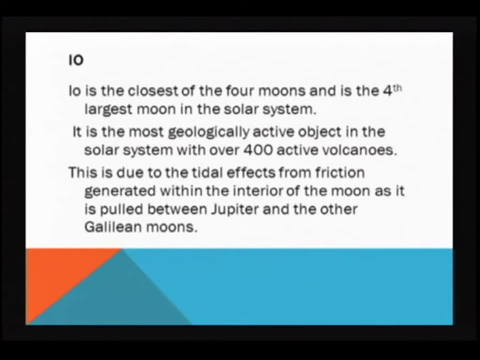 in every direction you possibly can think of, and then you get off. Now, what are you going to feel like Now? my guess is you're going to be a little sick to your stomach, and my guess is you might want to go find the nearest restroom and throw up. 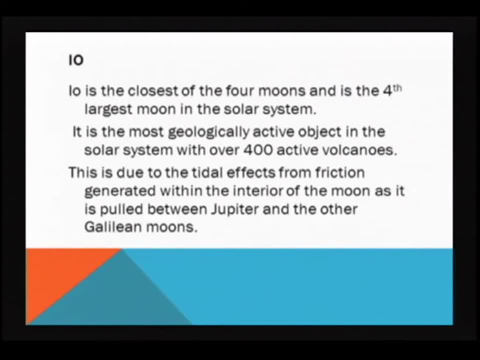 Well, guys, that's exactly what's going on with Io. Only, instead of, you know, having the rides, you've got Jupiter, which has an extremely strong gravitational field and an extremely strong magnetic field, And Io is basically getting pushed back and forth. 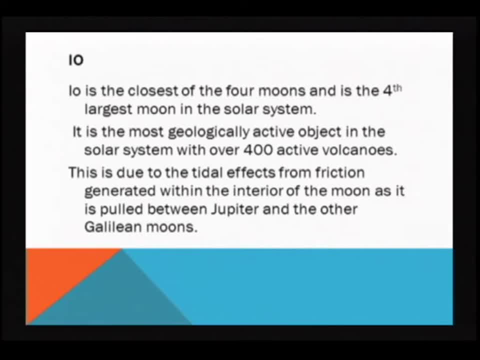 and jumbled up from tidal forces, from the friction generated between the interior of its moon and the gravitational pull between Jupiter. You know, you just get all these forces that are impacting and just like what your stomach's going to feel like after you get off of those rides. 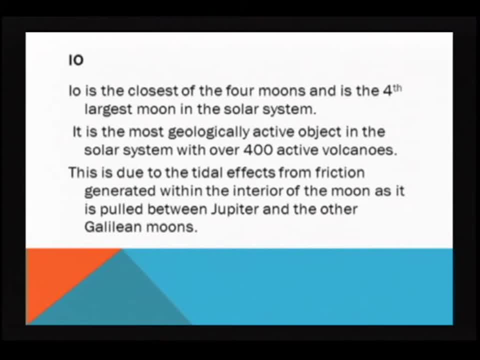 well, that's what the insides of Io feel like, you know. So it is churned up completely and therefore it's spiraling up. It's spewing volcanoes all over the place. Now we're going to find that the other moons. 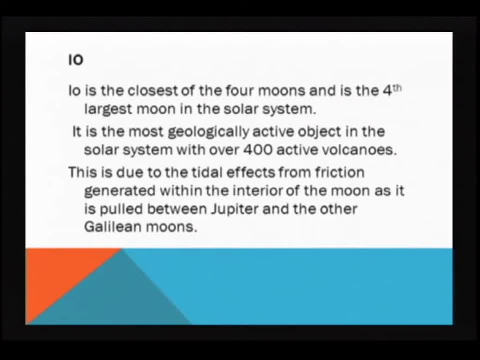 the Galilean moons- at least the next two- also have those tidal forces at work, but they show up a little bit differently. Io is so close that Io gets basically a lot of that, And so you have these volcanoes that are produced. 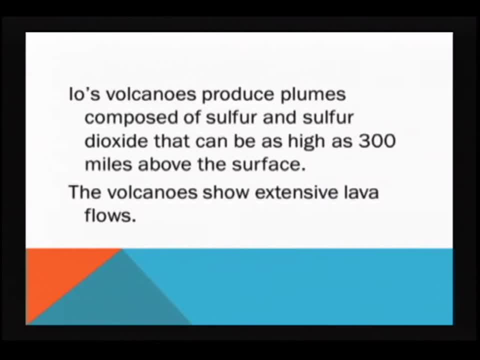 because of that, so it continually keeps it churned up. They produce these incredible plumes of sulfur and sulfur dioxide. You've got these really cool oranges and browns and yellows and blacks And notice those plumes can be as high as 300 miles. 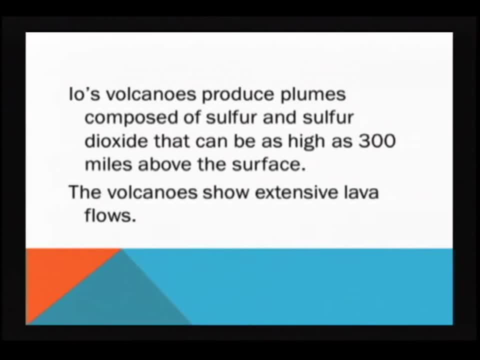 above the surface. We don't have anything like that here on the Earth. And number one, Io, is much, much smaller than the Earth, so its gravitational field is less, so you certainly would expect these things to be higher, But these things look really cool. 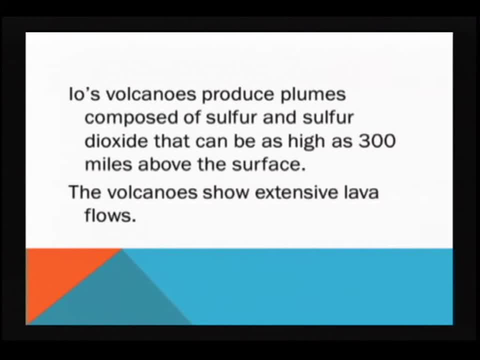 because you don't have the type of atmosphere that we have here on the Earth, and so they go up And they just come down like these incredible fountains, And then, when you look at the surface, you're also going to see extensive lava flows. 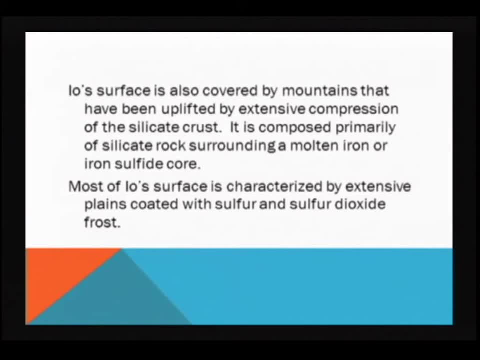 We know Io's surface is also covered by mountains that again have been uplifted by compression from that silicate crust. Again, thinking about those tidal forces that are acting on Io, Composed primary of silicate rock, kind of expected. 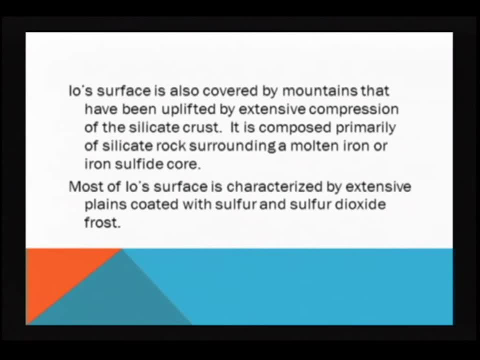 and you've got that molten iron or iron sulfide core- But notice the word molten in there- because those tidal forces are keeping that material liquid. Most of Io's surface is characterized, like I said, by extensive plains coated with sulfur and sulfur dioxide frost. 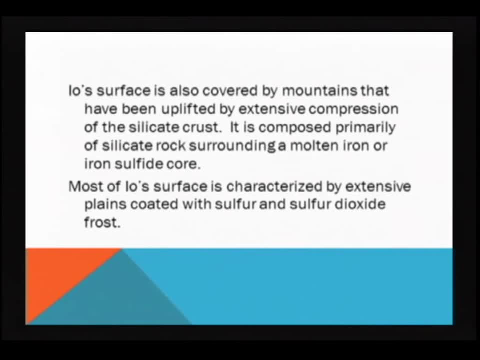 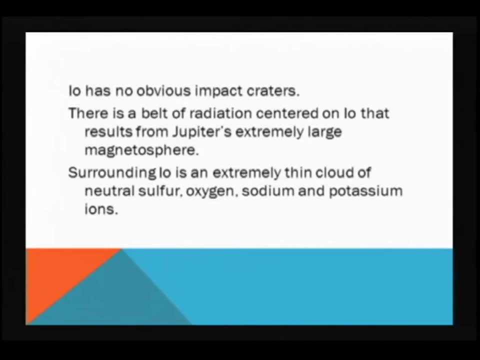 So we can actually see that frost on that surface. No impact craters that are obvious. Does that mean they never had them? Of course not. It just means that those impact craters that occurred were simply destroyed so very quickly by all the volcanoes that were going on. 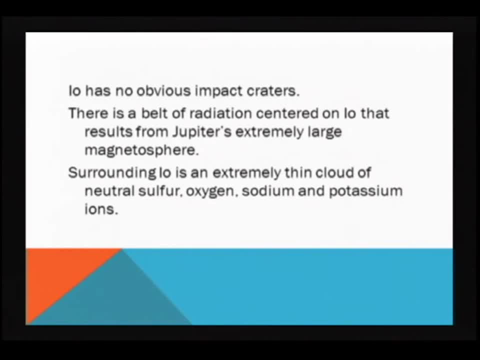 And that's what's going off on Io. We also know there's a belt of radiation that's centered on Io, that's coming from Jupiter's really large magnetosphere, basically Jupiter's magnetic field, And that's going to be true of Io as well as some of the other moons. 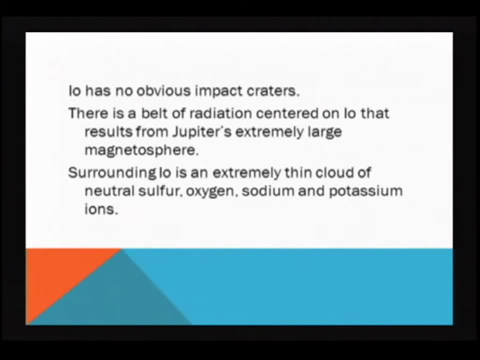 And then surrounding Io, it's not so much an atmosphere as it is material that has been thrown up from the volcanoes, And it's a thin cloud of neutral sulfur oxygen, sodium, potassium ions, things like that- that have been given off from the material. 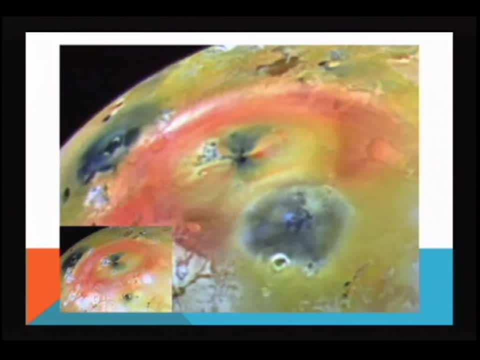 that comes up with the volcanoes. So this is a picture of Io. When the original pictures came back from Io, people called it the pizza moon. So I want you to think of a pepperoni pizza with some sauce around there, some cheese around there. 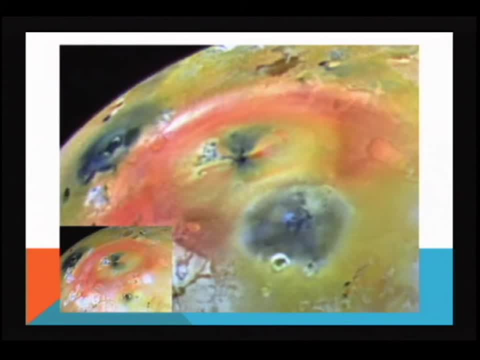 And so you're seeing these big, huge volcanoes that are active, that are going off, And if I look at this picture, you can certainly see that there's evidence of lava flows. That's what the dark area is. There's certainly evidence of active volcanoes. 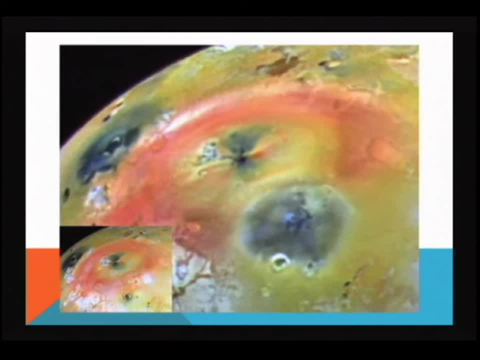 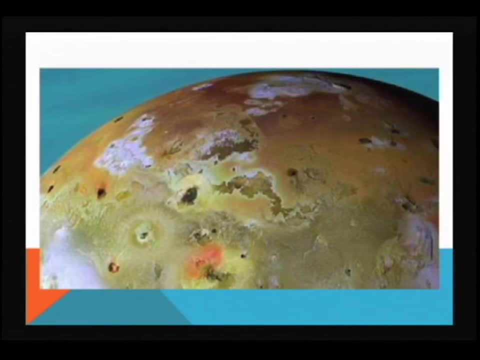 That's what that kind of reddish material is. We can see lava flows, So we got closer. there We're going to see some actual lava that is flowing. Another picture of Io. See some of that white areas are the frost. Remember it's not water. 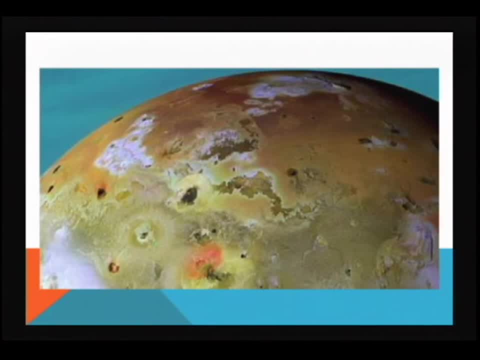 It's frost. It's a chemical-type frost, But you can see where those old lava flows have been And you can see how many volcanoes are on the surface there. You've got an active one where that red is, down there at the middle bottom. 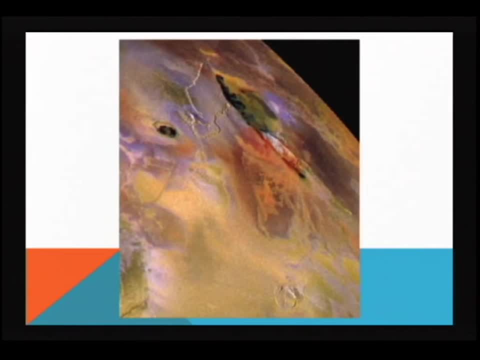 and then you've got one over there on the left. That's another picture of Io showing active volcanoes. That's got to be a really cool place to go around. Don't know that I actually want to land on there. First of all, I'm not sure how much of that surface there is. 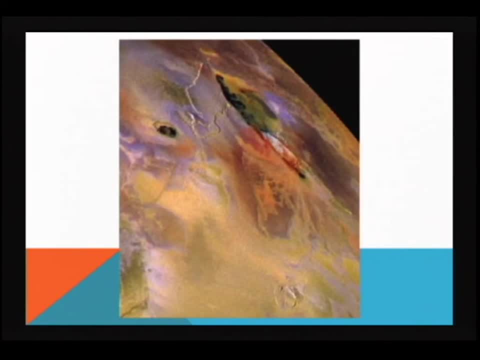 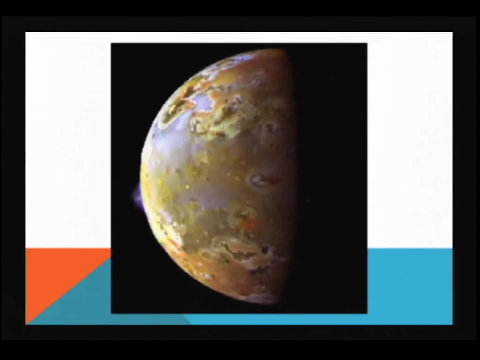 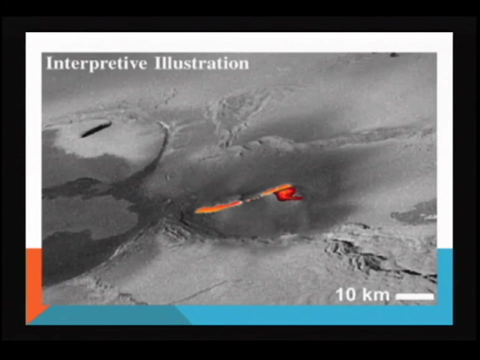 This is really solid as opposed to liquid. I mean, doesn't that look like a pizza? Here on the left you're seeing one of those plumes, And then we're actually looking now at the surface of Io Because, remember, we've got the Galilean probe out there. 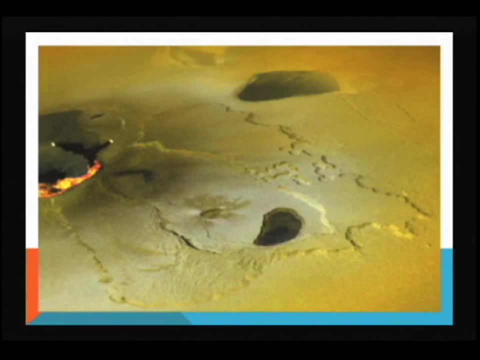 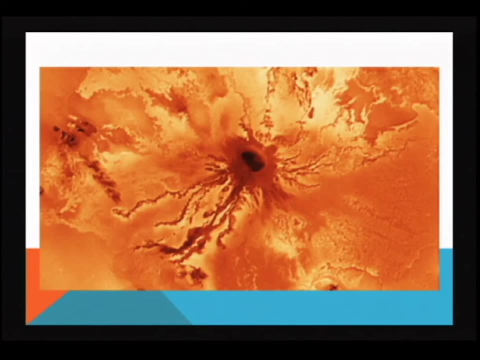 and so we are able to get really nice good close pictures of Io, as well as the other four- Excuse me- the other three. It's a really nice active lava flow right there. Now this is a false color. 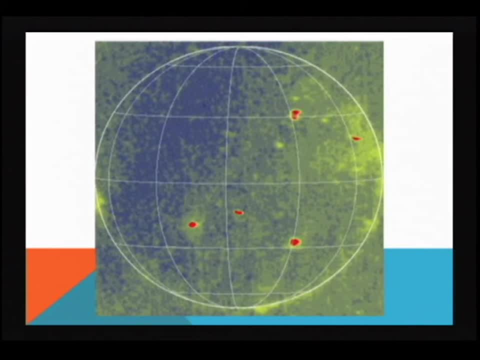 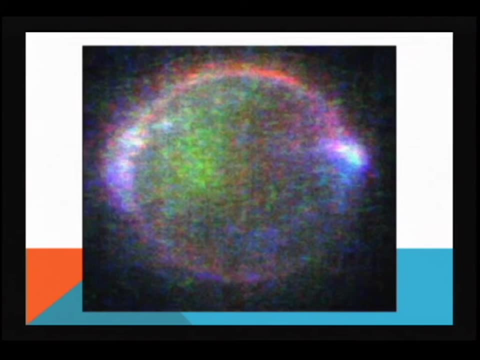 and this is looking at Io under intra-red light, under heat, and so you can see those active volcanoes right there. And then this is kind of that plume that I was talking about. This is obviously not visible light, guys, You know, and it's colored that way to go ahead and bring out. 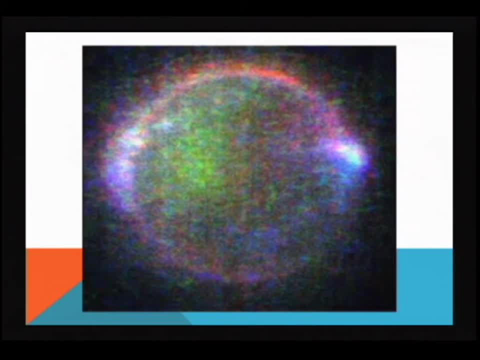 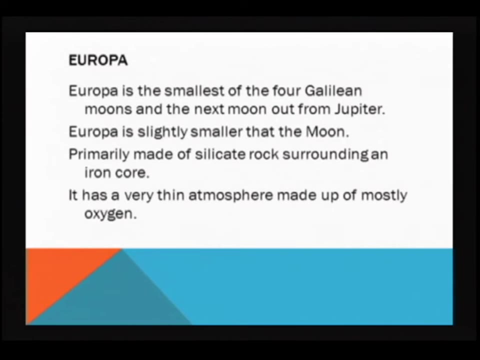 the different chemicals, But that's that kind of material that's in orbit around Io being kicked off. So now let's go from Io to Europa. Europa is the smallest of the four Galilean moons and it's the next moon out from Jupiter. 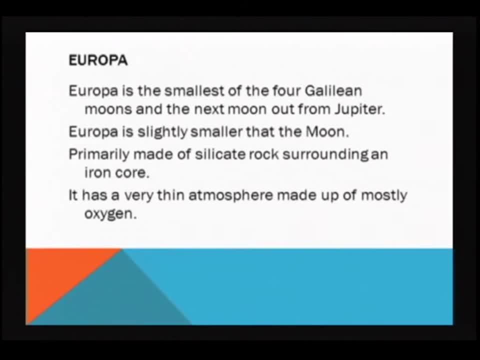 It's slightly smaller than our moon, primarily made of silicate rock surrounded by an iron core. Now it does have a very thin atmosphere made up of mostly oxygen. Now, Europa, as opposed to Io, Europa's surface is covered by ice. 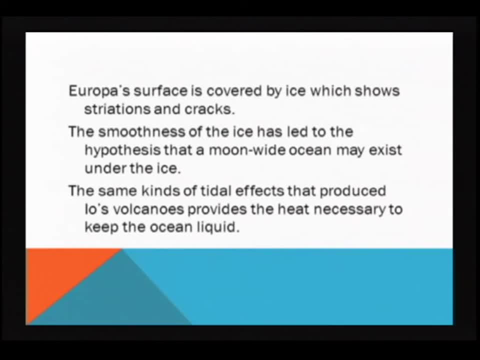 and that ice shows stridations and cracks and things like that, And the smoothness of that ice tends to make you think that maybe there's a moon-wide ocean that is interacting with Jupiter's magnetic field. We also think that moon-wide ocean. 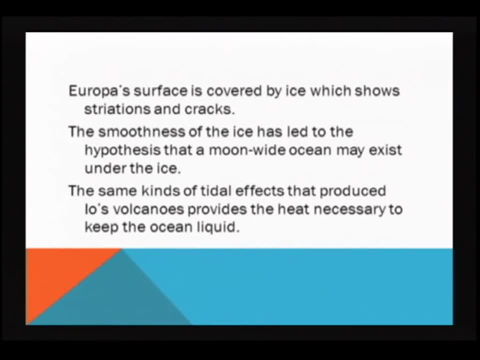 there might be a possible place for life. You know, the same kinds of tidal effects that we saw on Io, that produced all those volcanoes, are still working on Europa. but now Europa's far enough out, the surface of Europa has cooled. but that same internal mixing then. 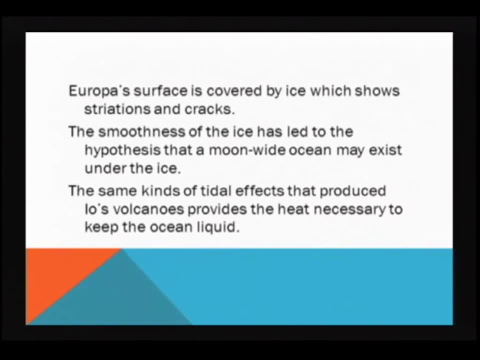 has kept that ocean as liquid as opposed to solidifying. So, even though Europa's out a little bit further and you don't necessarily see that those tidal forces are still working there, Now we can, and I'm going to show you some pictures of Europa. 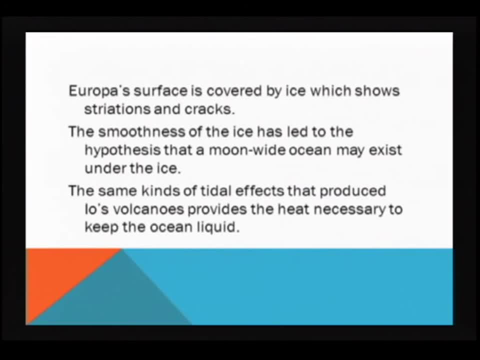 here in just a minute and you can see that it is indeed covered by ice, and you can see where it looks like it's sometimes split open, it's been hit, those kinds of things, And so, because it is so cold, it does immediately go ahead and solidify back. 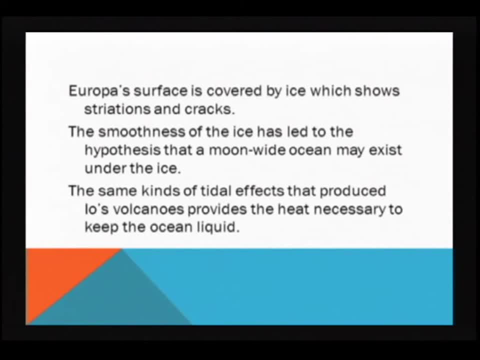 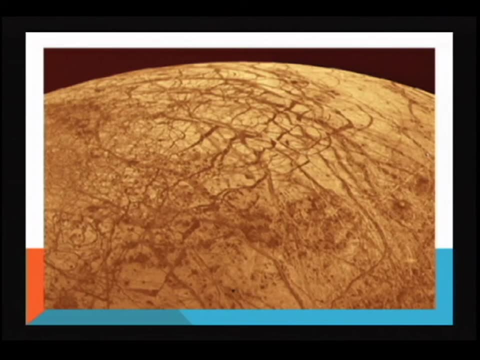 but then that means it protects the ocean that might possibly be under there. And this is a picture of Io. You can see some of the cracks there, but that's completely covered by a surface of ice. This just is a close-up. This just is a close-up picture of some of that ice. 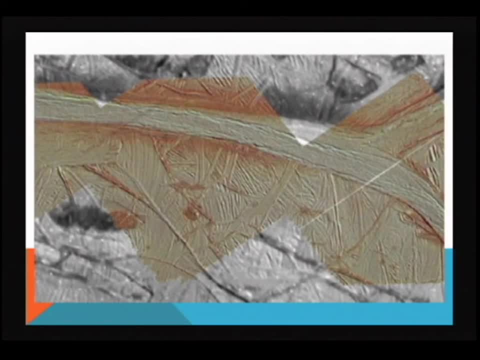 You can see where it looks like it's been hit, it's solidified, and then it froze back over again. You get that compression which sometimes causes the ridges in the ice which we see here on the Earth all the time. 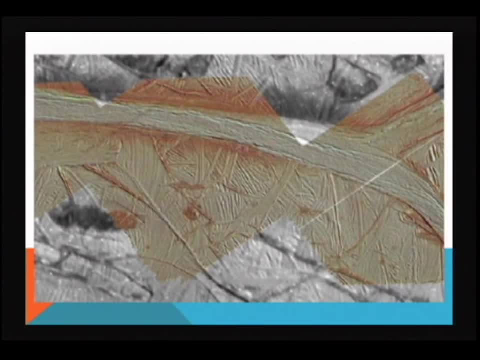 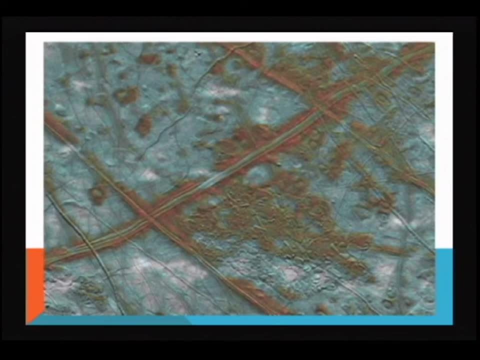 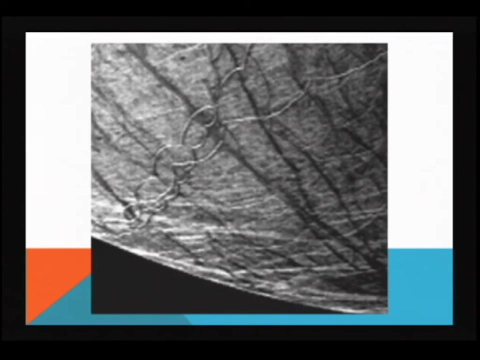 You know, you get those ridges formed as you get that expansion and contraction of the ice. It's another picture of some of the ice structures on Europa. Then we have things like this, Not exactly sure how they're formed, You know little ring structures. 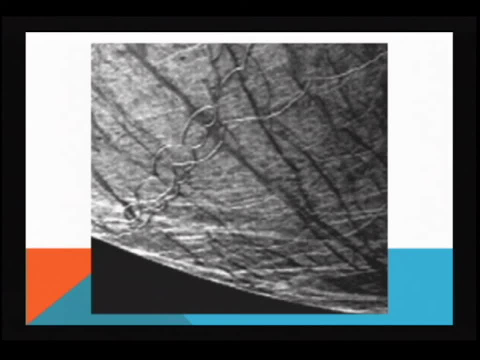 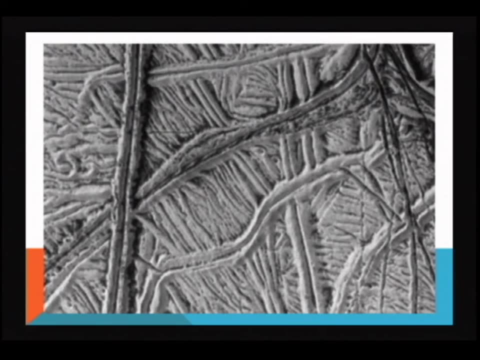 Actually have no clue how those things formed. Some of the ice that is whiter is probably a little bit newer. The darker ice is probably a little bit older, But the same kinds of mechanisms that we see occur with the ice here on. you know the Earth. 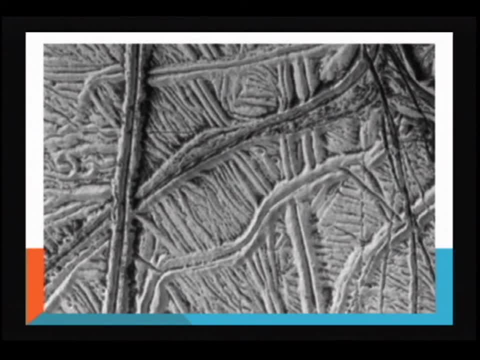 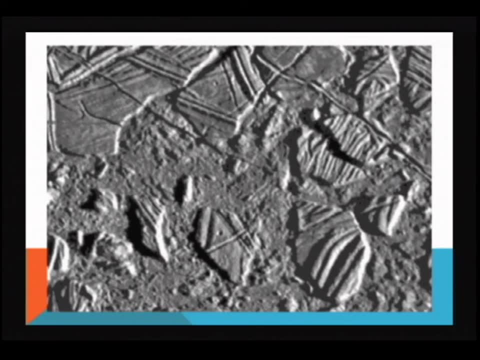 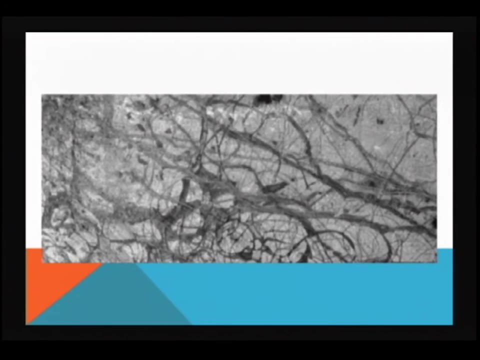 when a lot of these big lakes will freeze over, are the same kinds of structures that we see then on Europa, And again, expansion and contraction. I think that's kind of looking like a really cool abstract painting, But no, that's the surface of Europa. 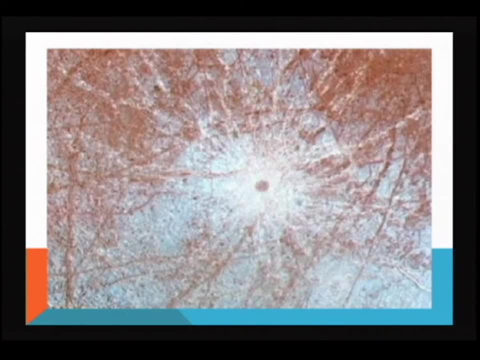 This is an impact crater on Europa where it probably solidified First of all, notice how white it is, So this is probably relatively young. Again, remember, I use the word relative And eventually that will go ahead and hit that same background color. 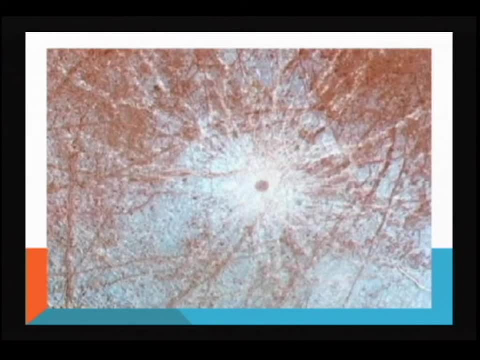 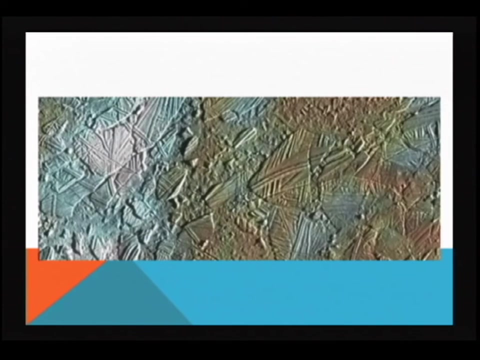 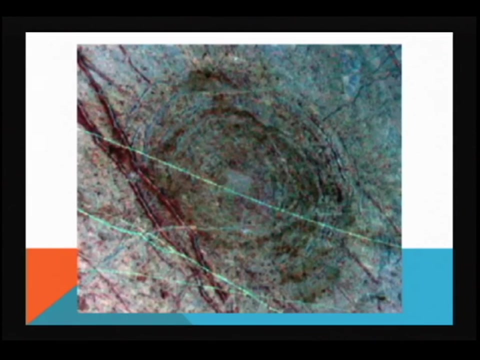 kind of that brownish, But it probably hit, probably broke the ice open, solidified that ice, then so cold that energy dissipated pretty quickly and it went ahead and froze back. Probably a very interesting place to go, simply because of the possibility of what might exist within that ocean. 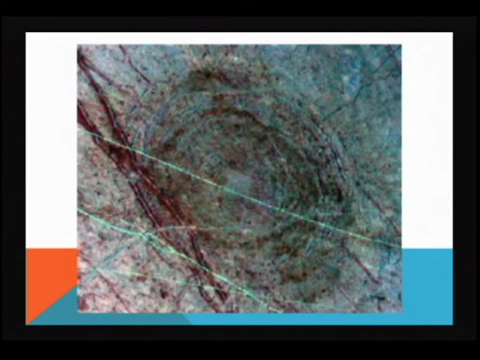 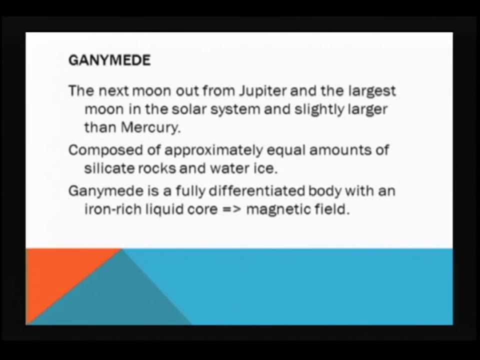 It's another impact crater. In fact, you can see those kind of shock lines and that solidified ice there. And then we had Ganymede, and that is the largest moon in the solar system. This one is slightly larger than Mercury. 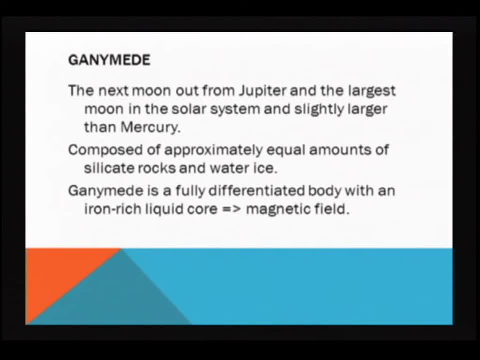 so our largest moon in the solar system is larger than one of our planets. It's composed of approximately equal amounts of silica, rock and water ice. It does seem to be a fully differentiated body, which means that you've got a core. 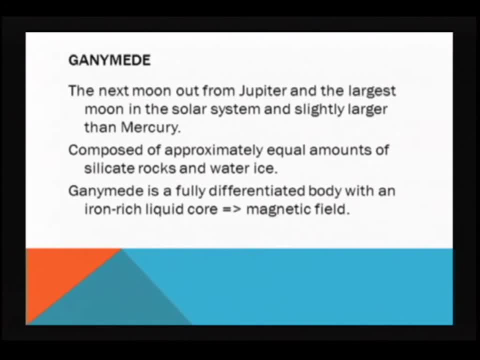 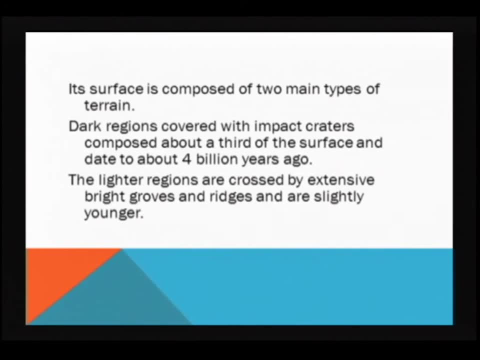 you've got a mantle and you've got a crust, And it does have an iron-rich liquid core, which means it does have a magnetic field. Now remember, it's further out from Jupiter, So those tidal effects are there, but at a much smaller amount. 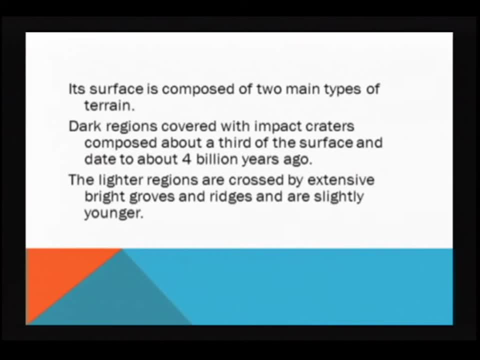 The surface does seem to be composed of two main types of terrain. you know lighter areas and darker areas, higher areas and lower areas. Those dark regions are covered with impact craters and they compose of about a third of the surface and date to about 4 billion years. 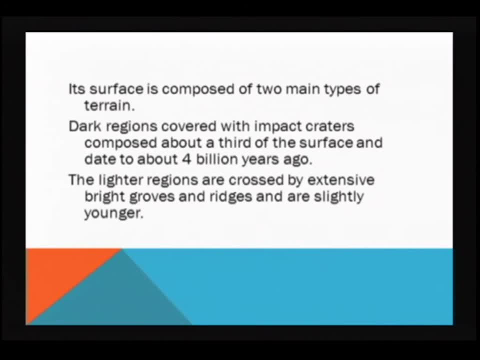 So that means something you know, since we know that it's about 4.5, 4.6 billion years, You know. so it has solidified and you've got those and lots and lots and lots of impact craters on it. 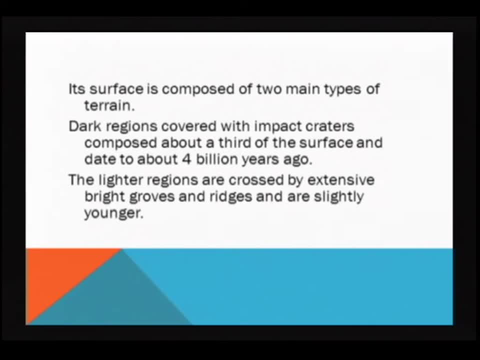 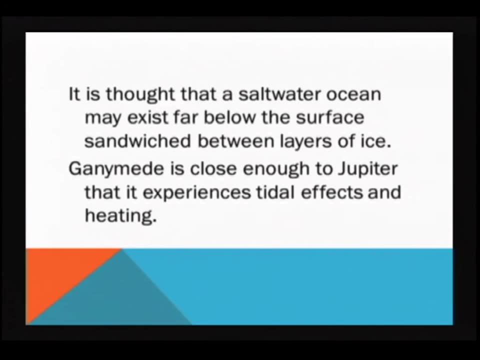 And the lighter regions are crossed by extensive, bright grooves and ridges and seem to be a little bit younger. Just like Io, just like Europa, Ganymede is still, as I said, affected by those tidal forces, And so we may. we think that there might be. 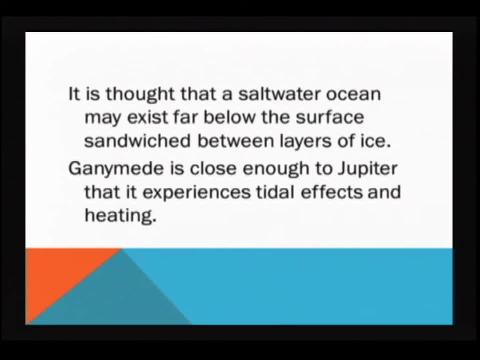 just like on Europa, a shallow ocean a little bit smaller on Ganymede than what it probably is on Europa. that's below the surface and maybe sandwiched between layers of ice. Again, it's not. we're not real sure. 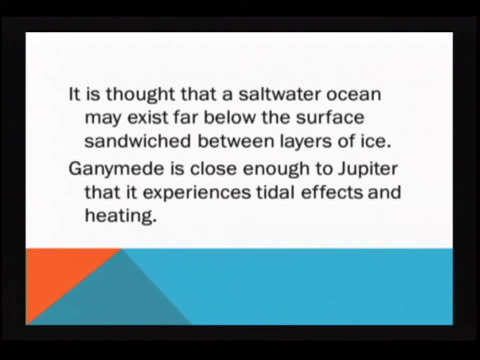 I mean, we're not out there, And we certainly do have Galileo, the probe that is out there sampling things, But you know, we still don't know a lot. A lot of this is still conjecture. We certainly want to go out and be able. 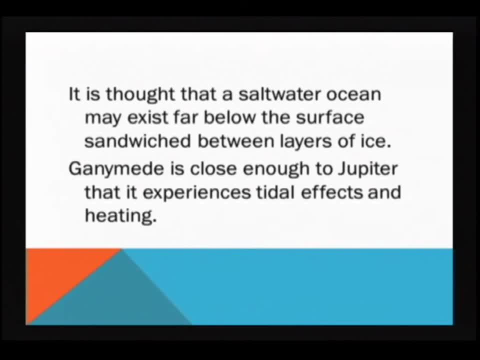 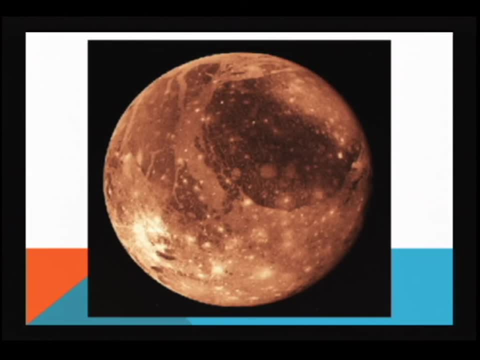 to visit those moons a little bit more, visit Jupiter a little bit more to really get a good feel for what's going on. This is Ganymede. Notice that really big, old, old dark area, How heavily cratered it is. 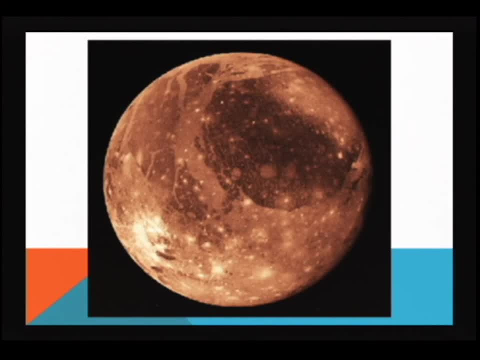 You can see some new craters down below. You see these bright spots. That's probably where something hit brought material up, and still very bright. We also might be looking at the tops of ice That is right under that. Remember we're out toward Jupiter. 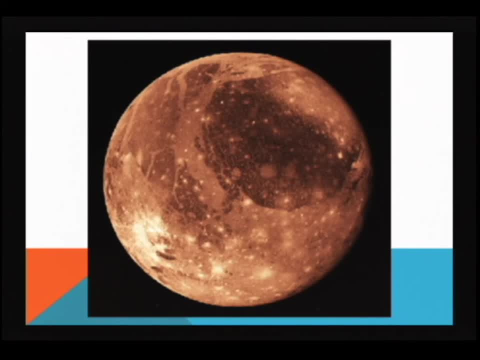 which means it's really really cold out there, And we do think that Europa, or Ganymede, does have ice in it, and so just hit far enough below the surface, it'll bring it up. We're going to see those same kinds of bright lights. 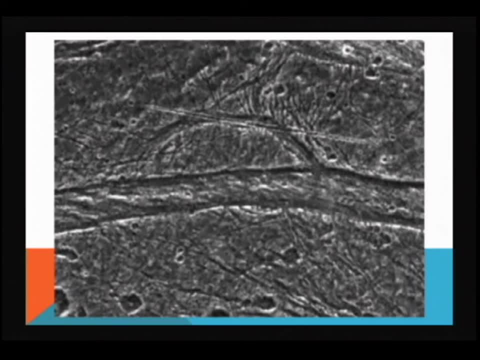 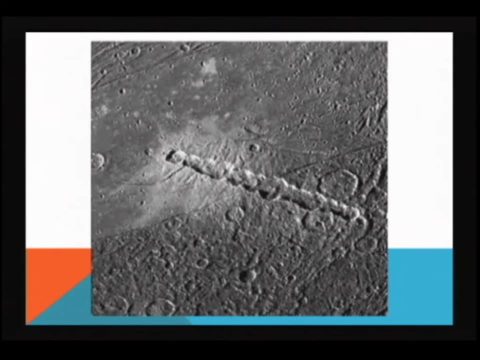 on Callisto. here in just a second, Just some more surface features of Ganymede. It probably looks more like your typical moon, And then you have the Mayflower or the Mayfly, excuse me, not the Mayflower, The Mayfly. 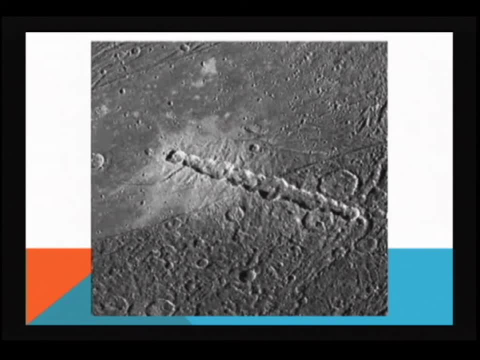 This is just a series of impact craters on Ganymede and brought up new material below, and so that's why you see the top of the, or the wing part of the Mayfly. It looks like a neat structure, but probably something came in broke apart. 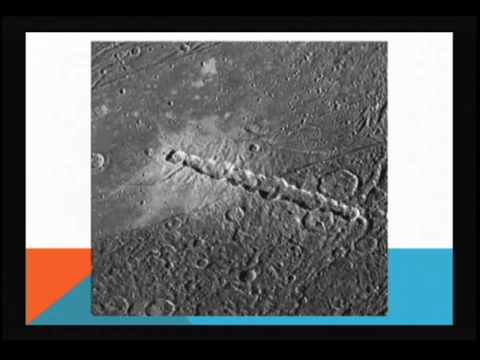 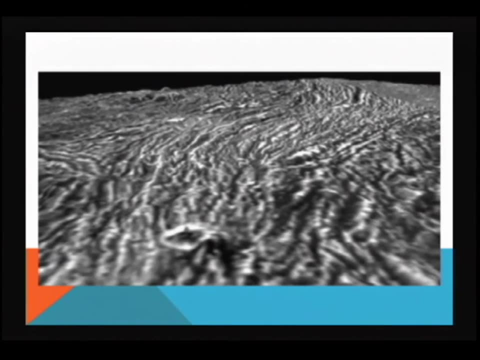 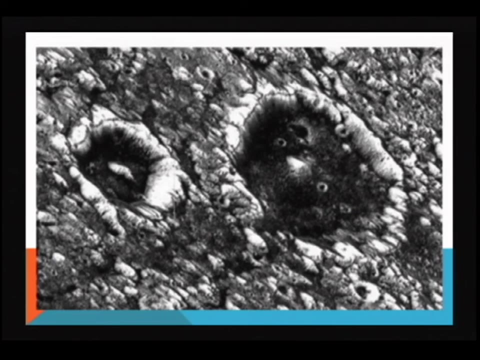 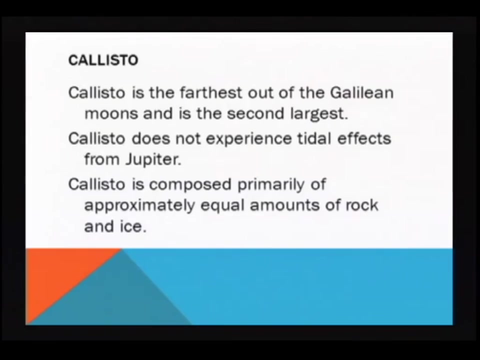 and just kind of kept hitting that as it hit the surface, And so we have what looks like a Mayfly. Just more pictures of the surface. Certainly impact craters- Typical things that you would see on a moon- And then you have Callisto. 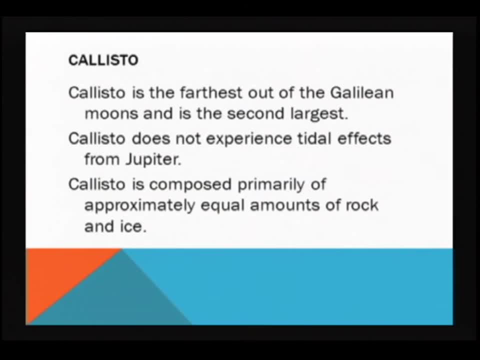 And it's the furthest out of the Galilean moons and probably the second largest, And it does not experience tidal forces. It's far enough away, that's not an issue, And it's composed primarily of approximately equal amounts of rock and ice. 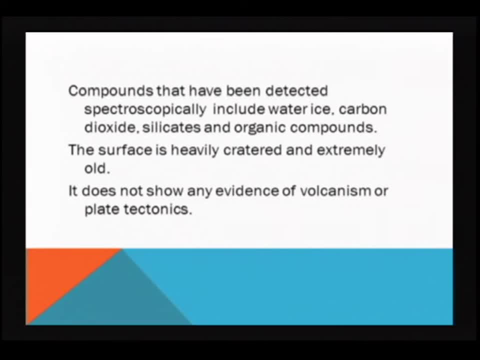 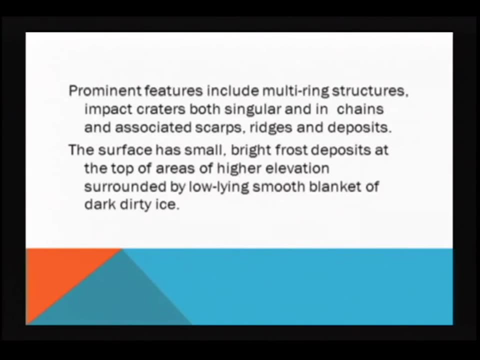 You know, we've seen carbon dioxide, we've seen silicons, we've seen organic compounds. The surface seems to be very heavily cratered and extremely old and does not show any evidence of volcanism or of those plate tectonics. 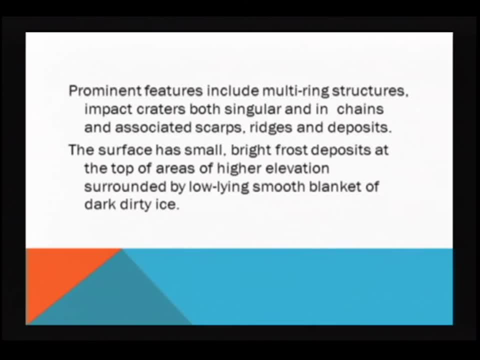 Primary features tend to include multiple ring structures. you've got impact craters. you've got them in single. you've got them in change. you've got all these scarves, ridges, all those kinds of things. The surface seems to have very small frost deposits. 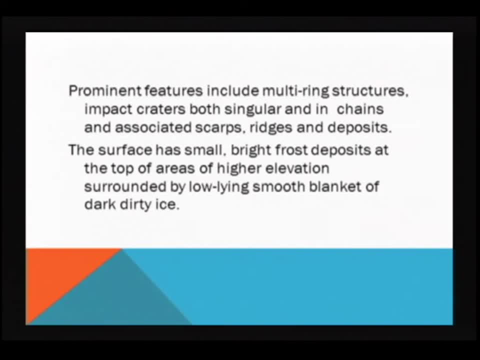 which makes it look kind of cool, because it looks like you have all these little lights there And then you've got that surrounded by this really smooth blanket of really dark dirty ice. Doesn't seem to have the same kind of core that. 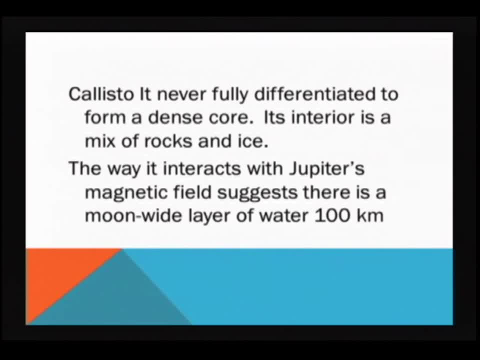 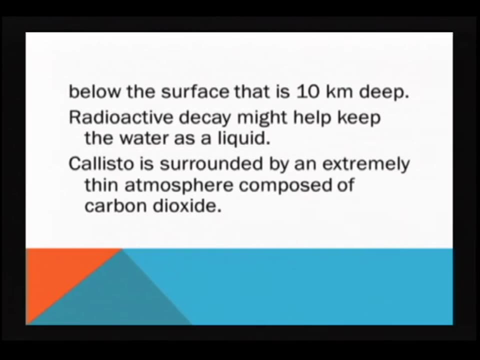 Ganymede has And again, the way it's interacting with Jupiter's magnetic field suggests that it may have a moon-wide layer of rocks, about 100 kilometers below and about maybe 10 kilometers deep, Surrounded by an extremely large, surrounded by an extremely thin atmosphere. 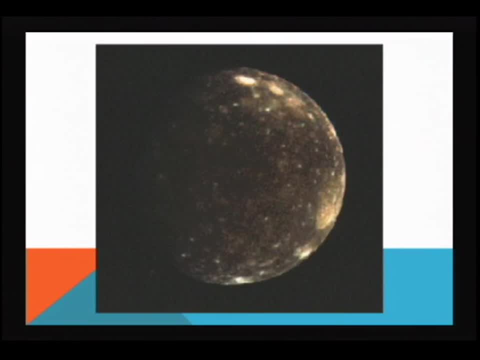 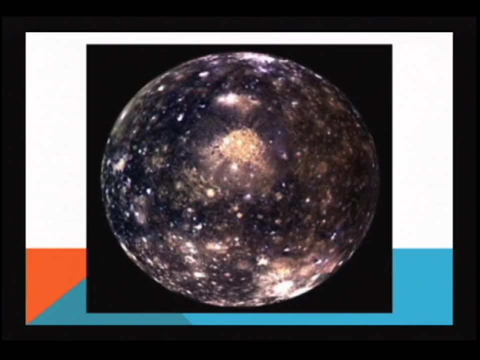 composed mostly of carbon dioxide. So here is Callisto, So those little bright areas, you're probably looking at ice. it's just below the surface, it's been hit and it simply hasn't gone ahead and weathered yet. 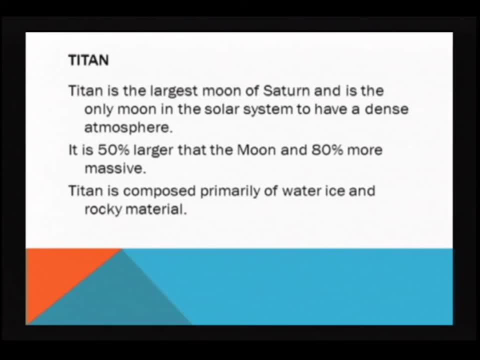 Other than that, it looks like a typical moon. And then we have Titan, which is the largest moon of Saturn, the only moon in the solar system to have an atmosphere. Notice, it's about, 50% of the time, 50% larger than the moon. 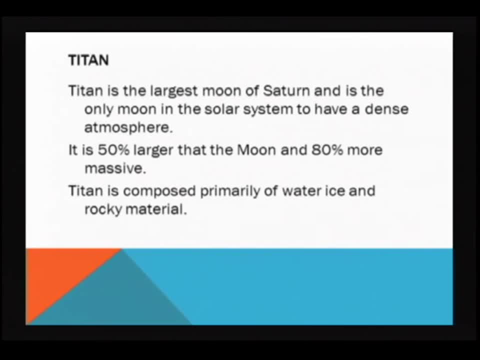 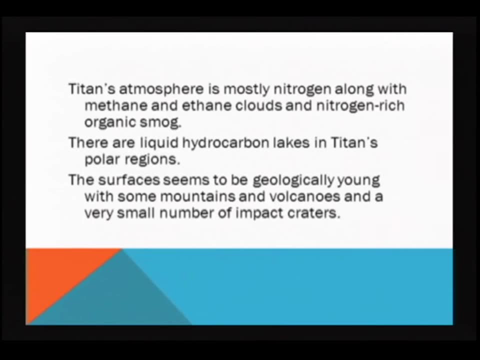 about 80% more massive, I think. it's probably composed of water, ice and rocky material. Seems to be mostly hydrogen, with some methane. I want you to think about our atmosphere with nitrogen oxygen and water dissolved in it. Well, methane is going to take the place of. 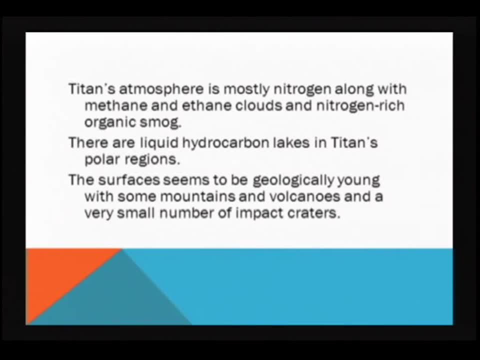 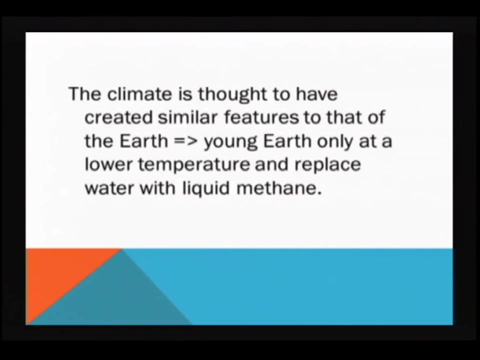 water in Titan's atmosphere, So we think there are liquid hydrocarbon lakes- seems to be geologically young, which implies that it's still geologically active And think about what the Earth was like when it was really young, and so we think that that's probably what Titan might be. 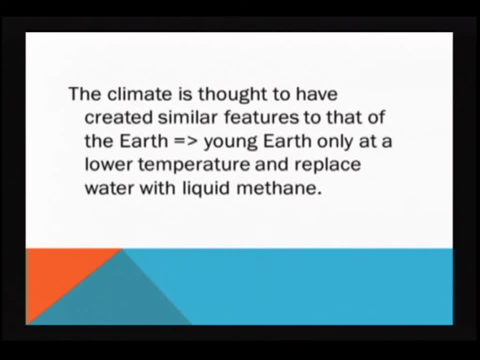 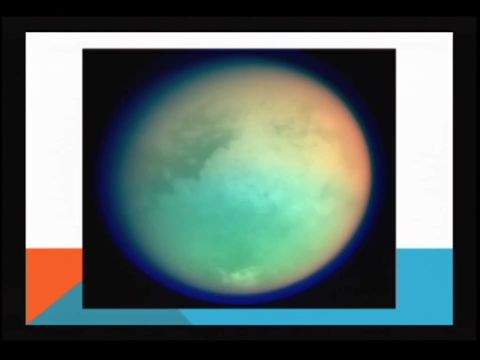 only with the fact that it's much cooler. and instead of having that nitrogen and oxygen mixture, you have then the other kinds of materials that make up the atmosphere of Titan, So liquid methane lakes, those kinds of things. This is a picture of Titan. 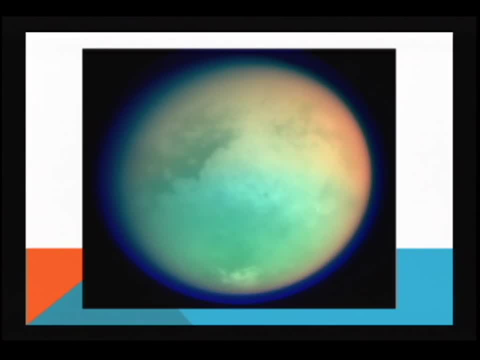 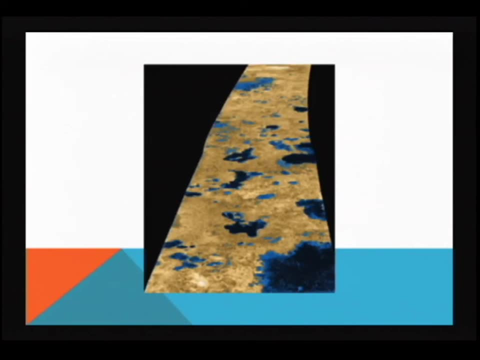 Notice. you can see, indeed, that layer of atmosphere around there. This is a radar map of the pole areas, and we think we're looking at those lakes that are formed from hydrocarbons. I said not water, but hydrocarbons. 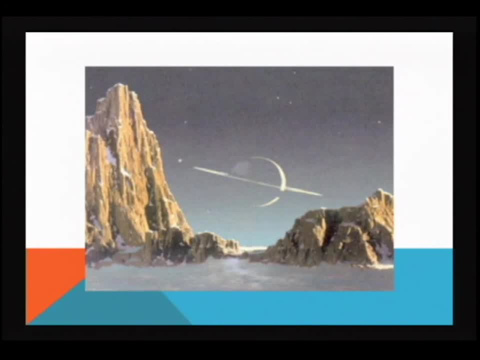 And this obviously, guys, is an artist's conception, but this is what Saturn might look like from Titan. That's got to be a phenomenal picture. Now there are all kinds of other moons, with both Jupiter and Saturn, Uranus and Neptune. 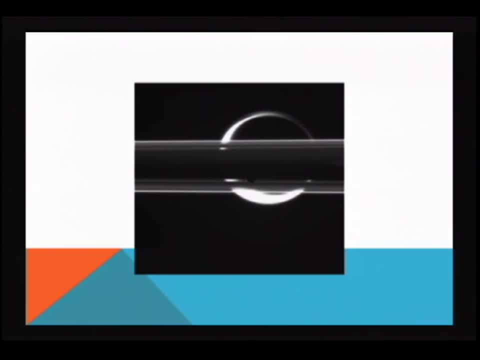 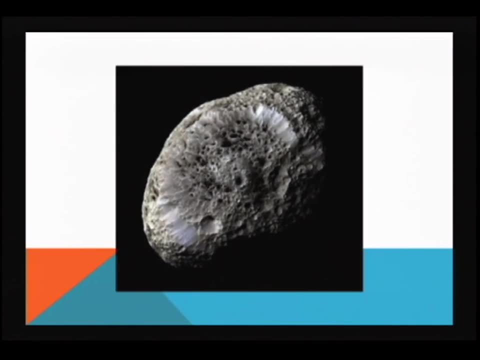 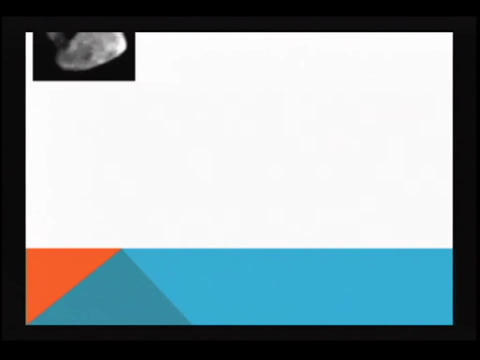 that we are really not going to talk about. but they have interesting characteristics as well. Most of them are probably captured asteroids. You know there's all kinds of other moons around there- Tend to be very small, tend to be very irregular. 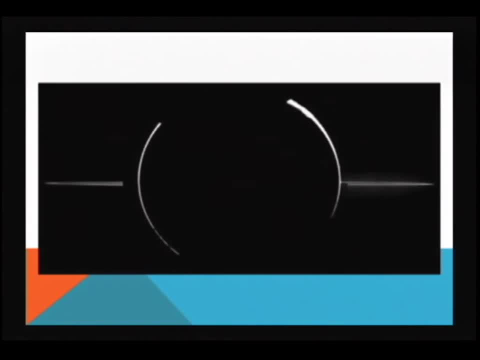 And then we have the rings in the solar system. Well, I've got a couple of pictures of the rings and we're not going to really talk about them right now because I have an activity that we're going to go ahead and look at these rings. 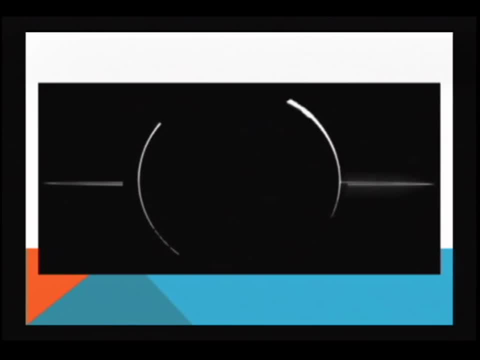 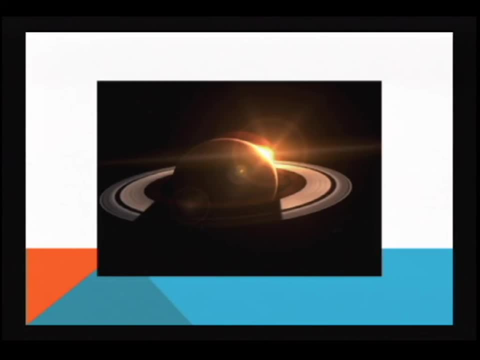 and look at how they're made, what they're made from, how they're kept in orbit. But here's the rings of Jupiter, Kind of dusty feel Rings of Saturn. I mean, there's over 150 separate rings of Saturn made of nothing more than dirty chunks of rock and ice. 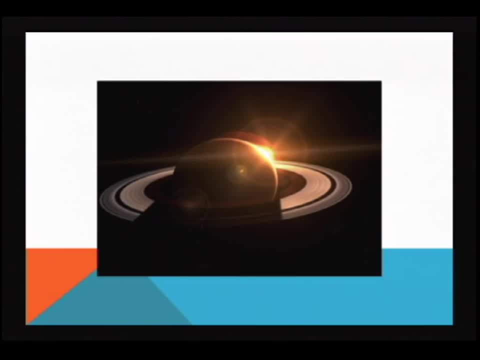 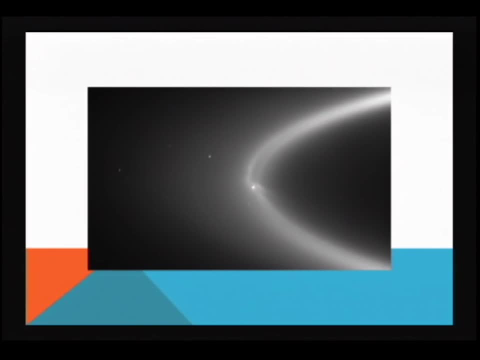 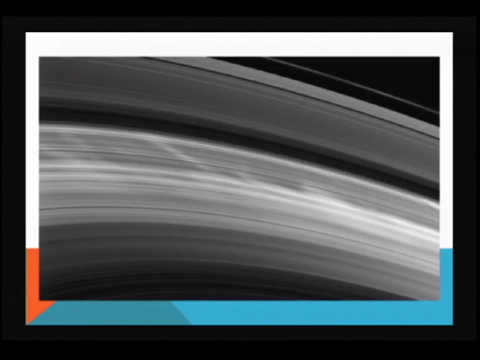 whereas Jupiter's rings are made mostly just of dark rocks and not so much of the icy materials. There are shepherd moons that are inside of the rings that tend to keep those rings in place, And then we have spokes that are in Saturn's rings. 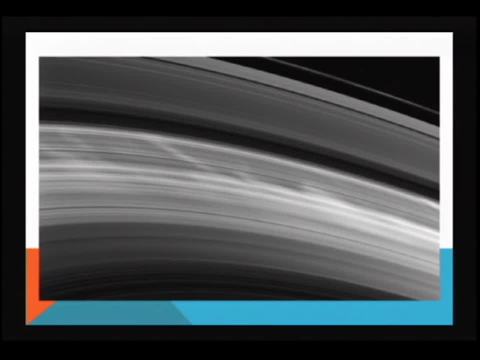 And exactly what those spokes are there for, how they manage to get there. how do they relate with the shepherd moons that are helping those rings stay in place? Not exactly sure, But, like I said, guys, we're going to go ahead and do an activity on looking at the rings. 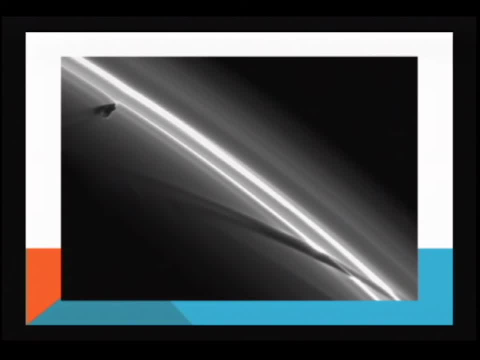 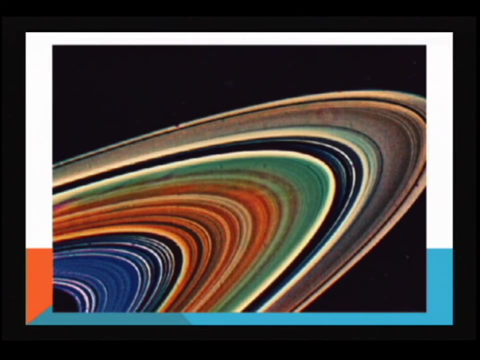 of Jupiter, Saturn, Uranus and Neptune, but especially concentrating on Saturn's rings and comparing Saturn's rings then to the other planets' rings. This picture of the rings of Saturn- Those are colored. that then help you look at some of the individual characteristics. 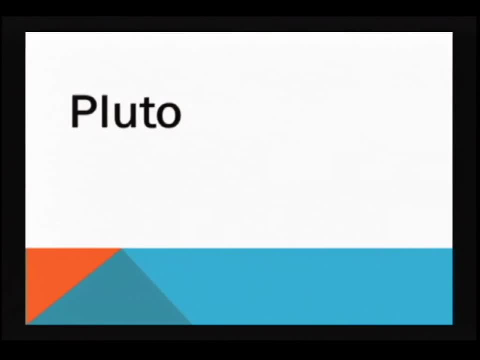 And then, guys, part of that activity that I have you do will center on Pluto And why Pluto is no longer a planet and why it's really a dwarf planet and what other possibilities are there out there that there are more dwarf planets. 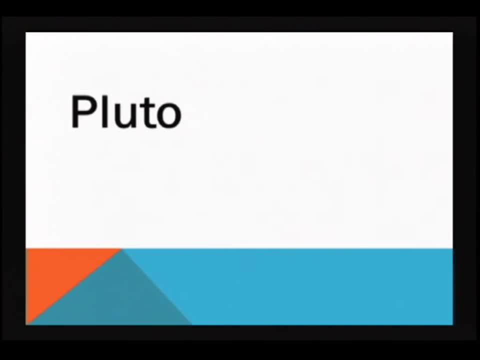 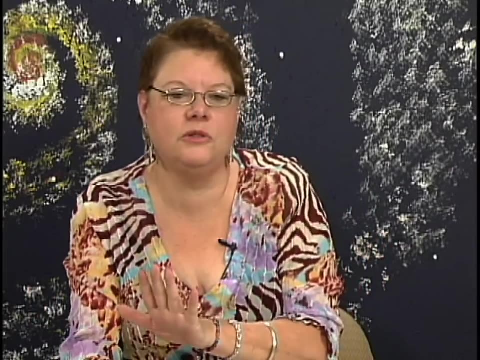 We certainly know there are, And what does that tell us about our solar system? So with that guys, we'll go ahead and, like I said, head to Blackboard and do a little bit more in comparing those moons, But this pretty well then will finish. 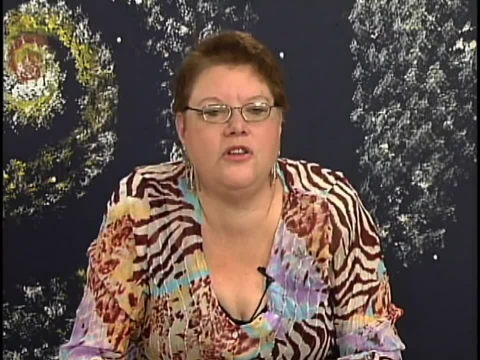 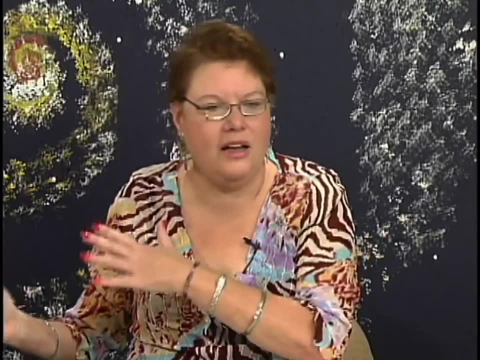 what I want to talk about, the moons today. Next time we'll go ahead and finish then our solar system with looking at asteroids and comets, And then we will head out from the Sun and on out to the rest of the universe for Unit 3.. 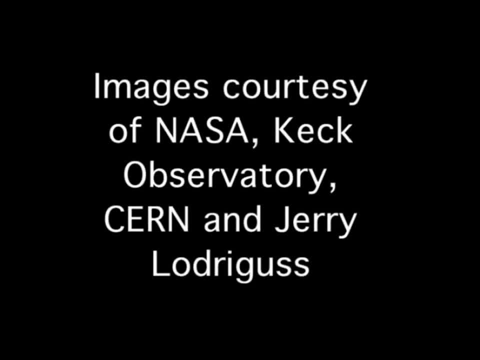 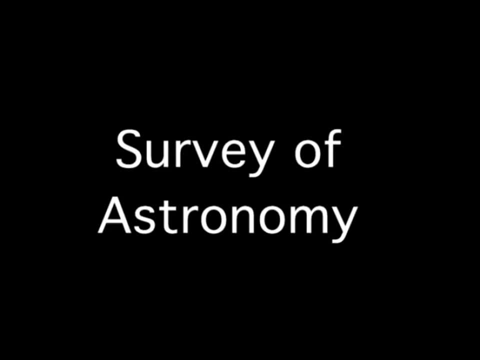 So see you next time guys.